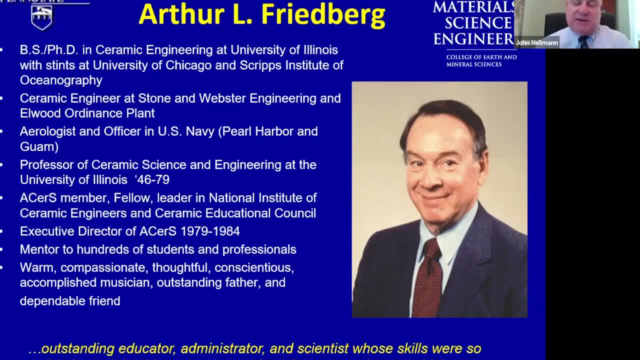 stint as our executive director from 1979 to 1964.. He's been a mentor to hundreds of students and professionals. He's been a very warm, compassionate, thoughtful, conscientious man, accomplished magician, outstanding father and dependable friend. Unfortunately, Art passed away. 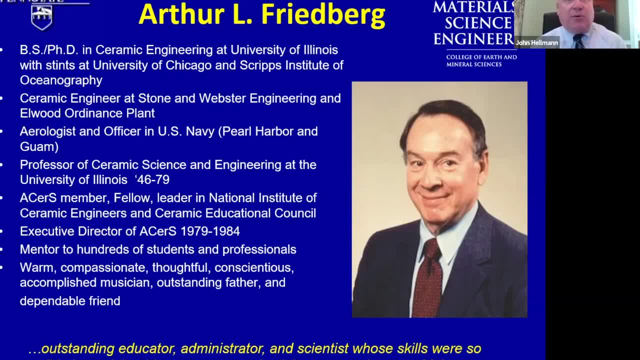 in 1984, but his memory lives on. In reading through his biographical information and so on, I came across numerous quotes and accolades regarding just how wonderful a man Art was. One really stood out one by one of our icons of ceramic engineering, Mal McLaren. He said: 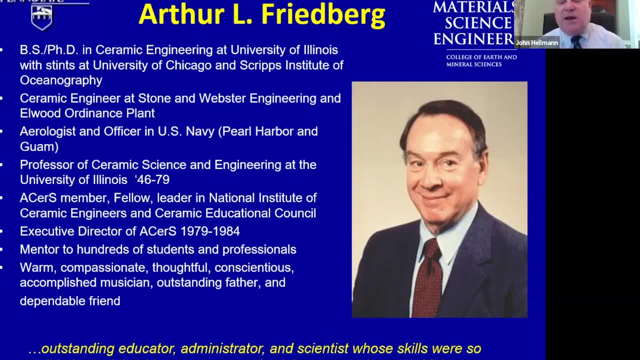 Art was an outstanding educator, administrator and a scientist whose skills were so well balanced that his enormous productivity appeared easy. That's a wonderful accolade, and it's in that spirit that I am humbled and honored to be able to give this year's Memorial Lecture. 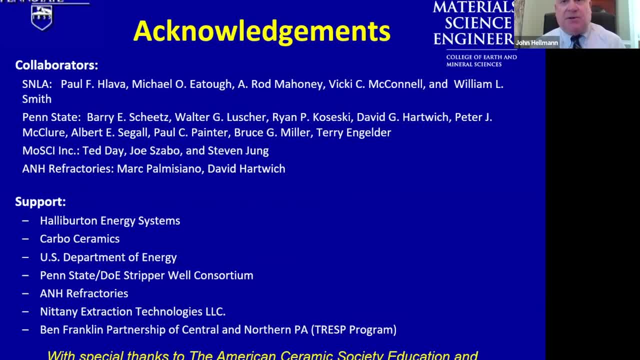 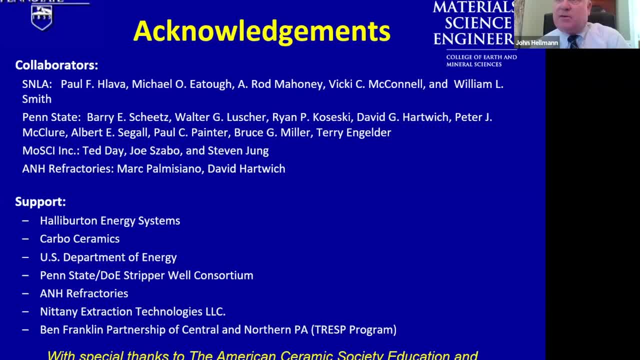 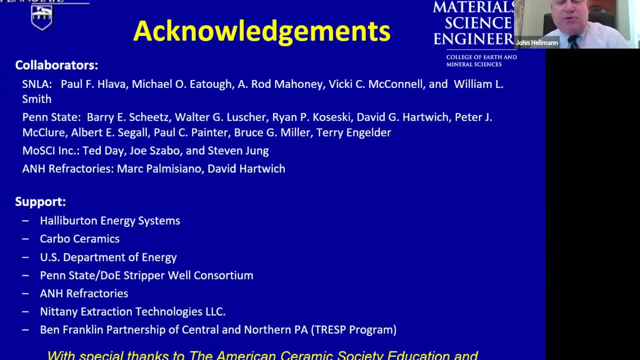 At Penn State. I collaborated with Barry Sheets, Bruce Miller, Paul Painter and Terry Engelder and my students Walter Luscher, Ryan Koseski, David Hartwich, Peter McClure and Al Siegel in the development of these materials and characterization of the processes and the like. 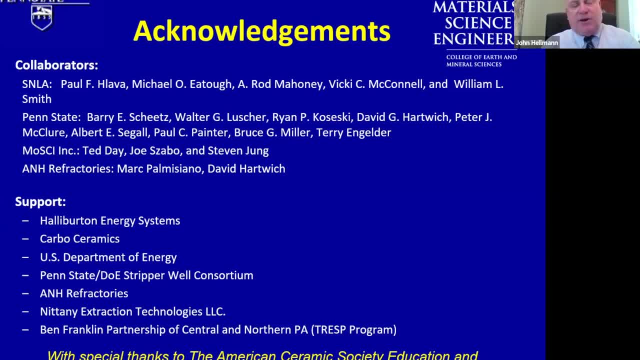 We had numerous industrial interactions, most notably with MOSAI, where we worked with Ted Day, Joe Szabo and Stephen Jung, and at ANH Refractories now Harbison-Walker, Mark Palmaciano and David Hartwich. 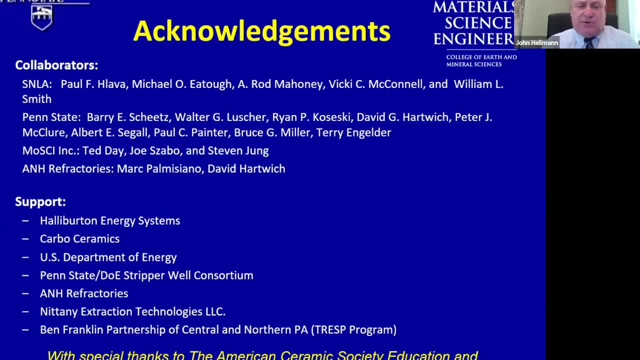 The support for this work came from a variety of industrial sources like Halliburton and Carbo Ceramics and Nittany Extractions Technology LLC, Harbison-Walker or ANH, and then from federal and state government like Department of. 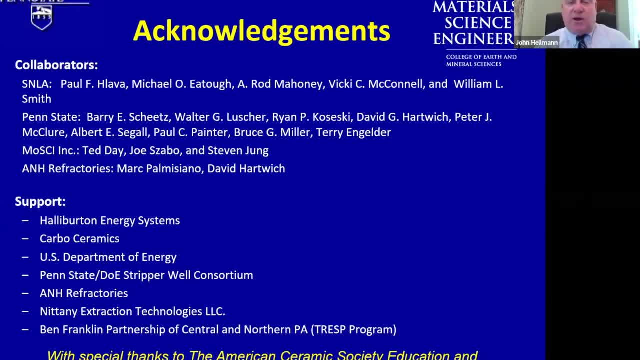 of Energy and the Ben Franklin Partnership of Central and Northern Pennsylvania, And it's with special thanks to the American Ceramic Society's Education and Professional Development Council that I'm here today to tell you about this work. Thank you very much. How did this work start? 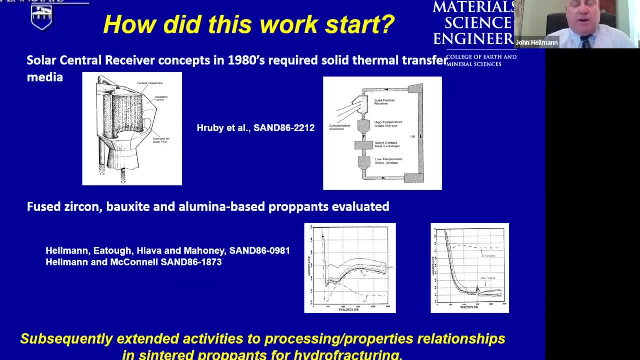 Early in the 1980s, while I was at Sandia, our group was tasked with finding a ceramic, solid thermal transfer media for a solar central receiver concept. In this concept, ceramic particles were to be dribbled through a insulating or a solar beam. 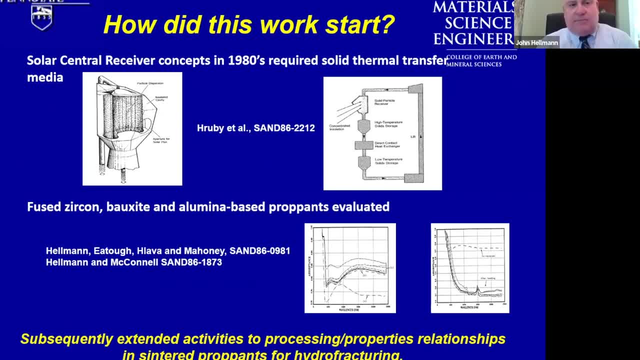 a concentrated solar beam that was derived from acres and acres and acres of heliostats or mirrors. This roughly 10-meter tall aperture through which the particles were irradiated yielded a residence time sufficiently long for the solar system to be able to transmit the energy to the solar system. 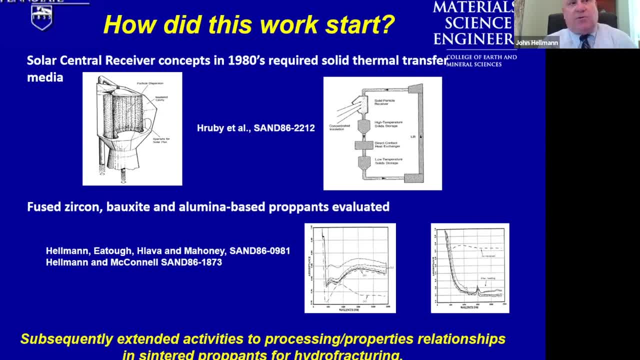 This roughly 10-meter tall aperture through which the particles were irradiated yielded a residence time sufficiently long for the solar system. This roughly 10-meter tall aperture through which the particles were irradiated yielded a residence time sufficiently long for the solar system, Such that the particles would increase in temperature from about room temperature. 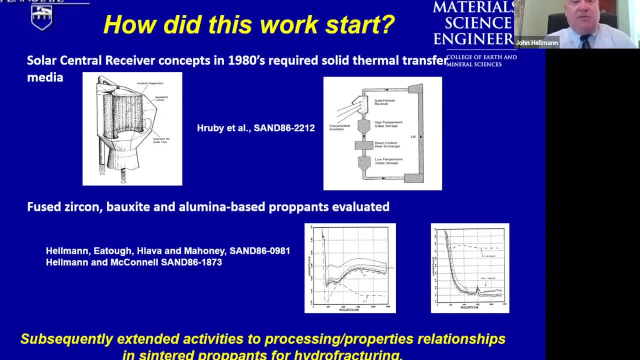 to on the order of 1500 degrees C, a very, very high intensity solar beam. These hot particles, then, would subsequently be stored and energy extracted from them to do industrial processing, such as cracking ethylenes, and then recycled through the system repeatedly over the lifetime of the system. 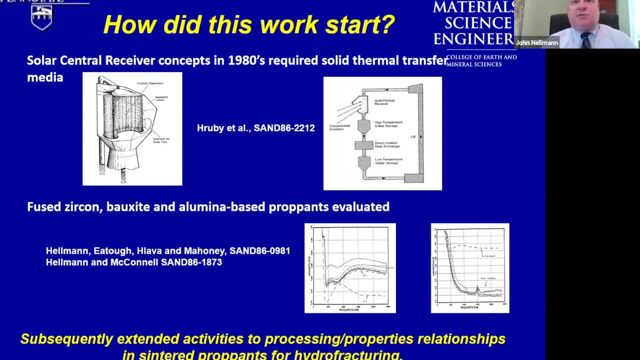 to capture the solar radiation, transform it into thermal radiation for industrial processing. The charge, the batch of ceramic particles that would go into this system- was on the order of 12 million pounds. That's a large volume of materials, so it needed to be. 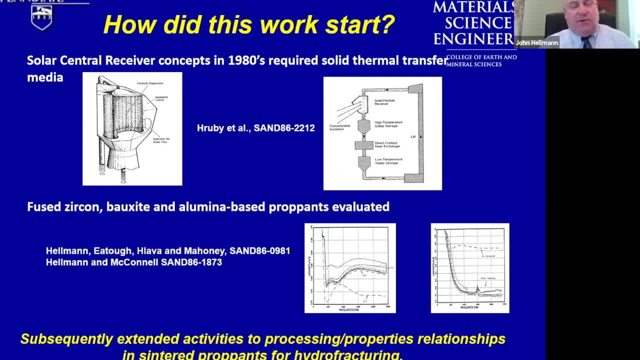 relatively inexpensive, obviously very refractory and mechanically and thermochemically robust to withstand repeated solar radiation. In this moment about 13 million говорит and ancritical materials industry And we examine particles that would be available for several bacteria. 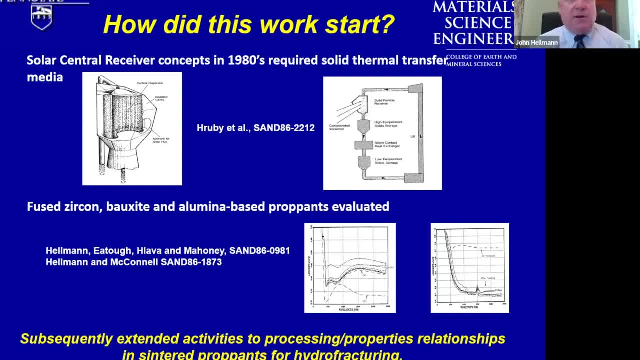 And we examine particles that would be available for several wear cycles over a lifetime of several years. We examine particles that would be available from the abrasives industry and there was no. we examine particles that would be available from the abrasives industry and there was no shortage of materials. 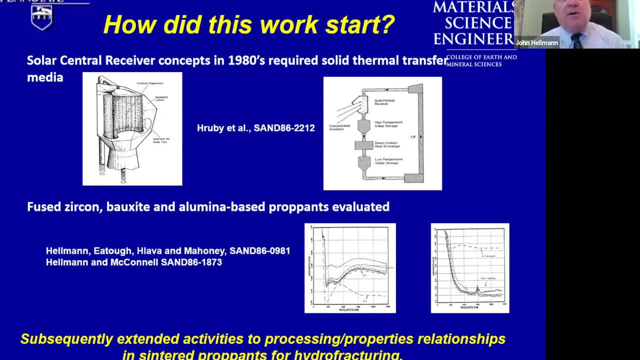 Due to the nature of abrasive particles, they were angular And the angular particles when they fell, the 100 meters through the solar central receiver during application and so on, would indent one another, causing cracking, which would contribute to failure and subsequently the generation of fines, which would increase the susceptibility of the materials, the particle bed, to sintering something you didn't want. 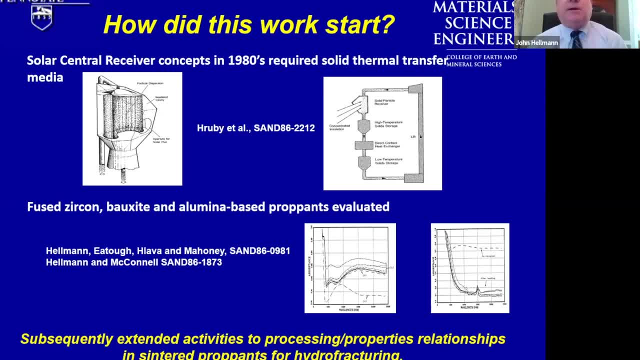 This bed needed to remain freely flowing for multiple recycling through the process. Therefore, we felt the need for using, or we determined the need to use, spherical ceramic particles. Spherical ceramic particles on the sizes necessary here, something on the order of a millimeter in diameter, were not readily available in the ceramic industry at the time, with one potential exception. 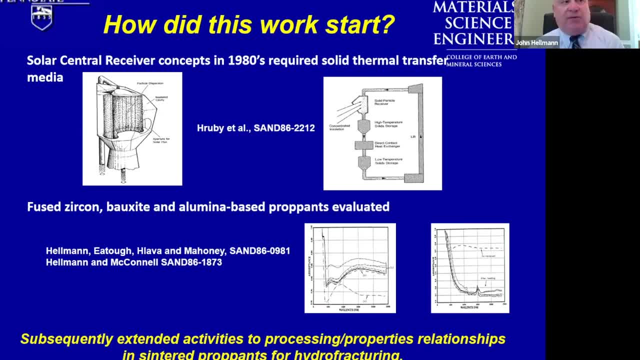 And that exception was A new family of materials that were being developed for the stimulation of gas and oil wells. These materials were known as propants. They were manufactured from ceramic materials in a spherical form and were becoming available on the market in the quantities necessary for use in the solar central receiver. 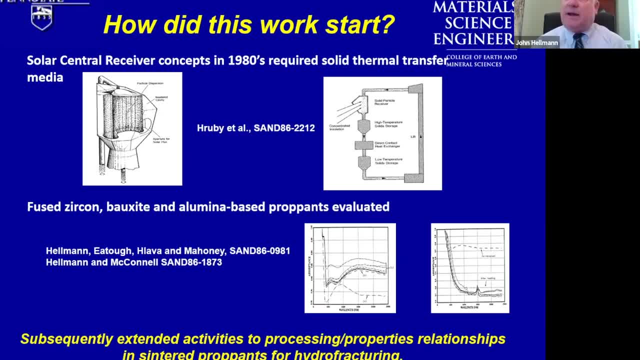 So we were able to demonstrate that technology and it worked out well, Absolutely, Absolutely, Absolutely. About that time I moved back to Penn State, started my work there on the faculty and decided that I would like to continue work on the propant materials for the oil and natural gas industry. and here's why. 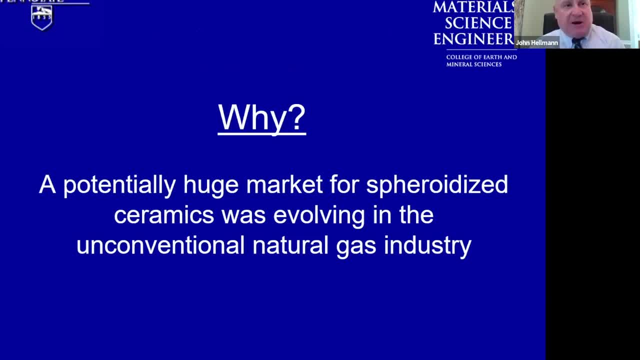 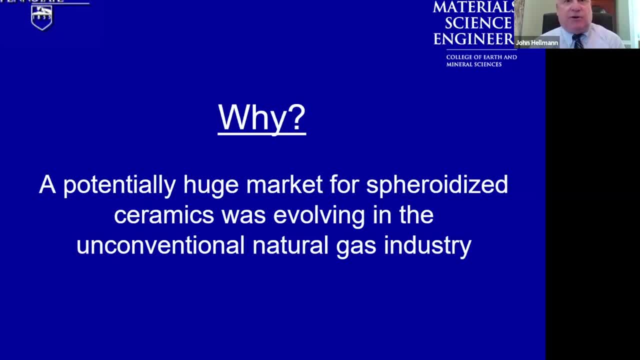 Evolving at that period of time was new technology, such as directional drilling and hydrofracturing, which was going to enable production of gas in a more economical fashion, from gas to oil that were not traditionally tapped in the past, because the vertical drilling technologies 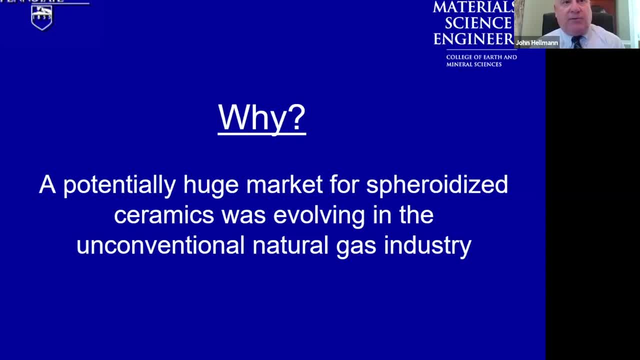 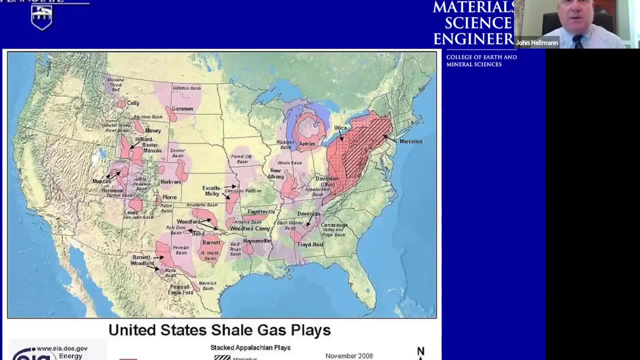 was just not appropriate for economic recovery of the gas. The horizontal drilling technology and hydro fracturing opened up these gas fields, some of which are shown here on this map of the United States. Now, some of these you've clearly heard about over the last 10 to 15 years. 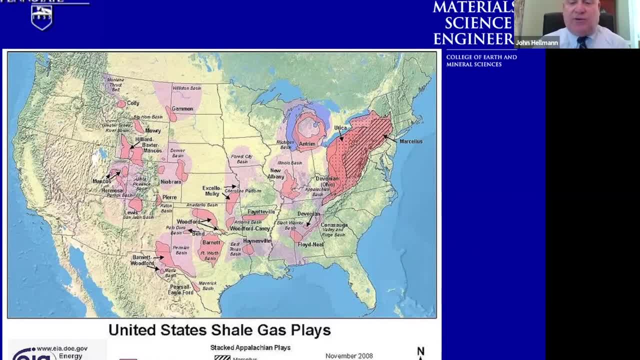 For example, the Marcellus Shale and the Utica Shales up in the Northeast of the United States. These gas fields contain sufficient gas to enable all of our energy requirements, to satisfy all of our energy requirements for something on the order of 150 years. 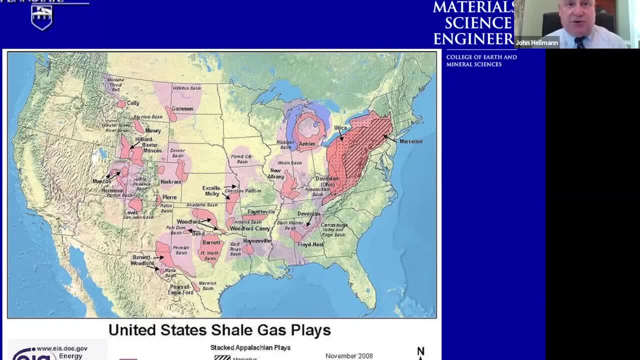 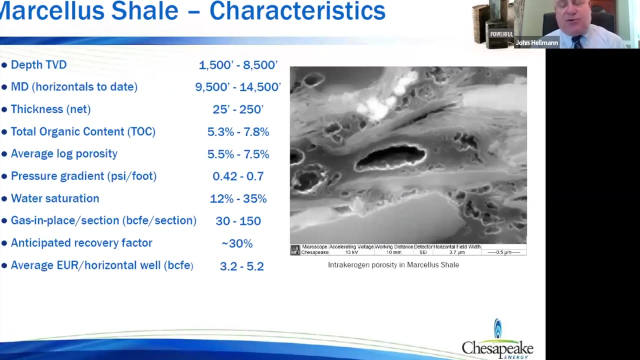 But we're only retrievable through the use and combination of several new technologies. Similar gas fields exist throughout the rest of the United States and indeed around the world. What this means is that the technologies need to evolve to be able to extract the gas from the porosity in these shales. 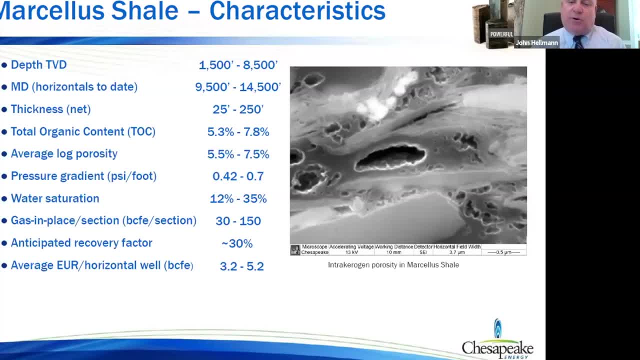 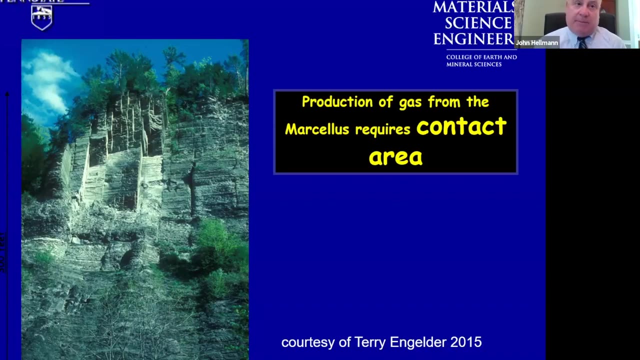 This is a picture of a Marcellus Shale, showing the pores in which gas is trapped and which you need to access during the drilling process via creation of new surface area- the whole purpose behind hydro fracturing. This shows a Marcellus Shale outcropping in New York. 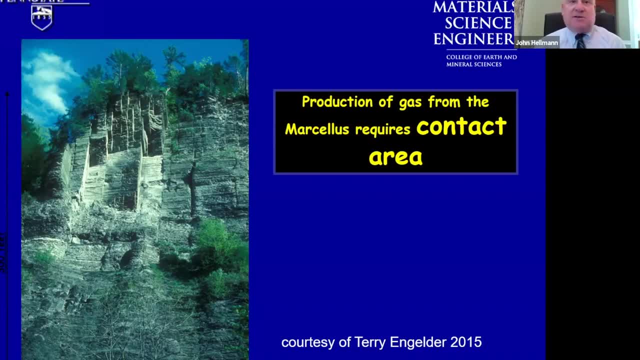 which you can see clearly the sedimentary nature of the rock or of the shale, as well as vertical fracture traces, which are common in the Marcellus Shale. These fracture traces are oriented roughly Northeast and Northwest. Those outcroppings that exist are essentially degassed. 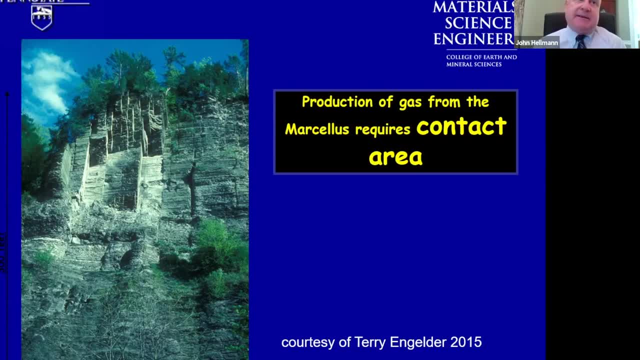 due to these vertical outcroppings and the like, And it's the deeply embedded shale and it's not just the deposits that we're after for production of natural gas, But the way you get to it is to create cracks in that shale. 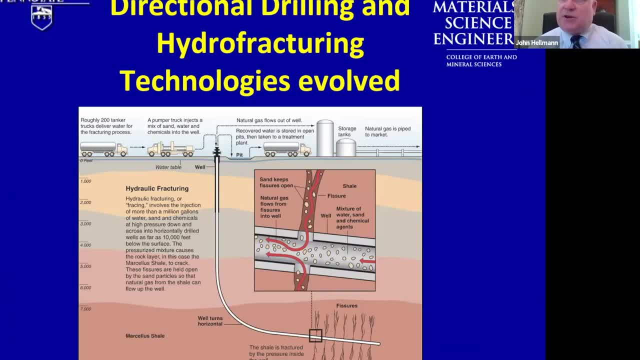 so that you can retrieve the natural gas using processes combining directional drilling and hydro fracturing. Directional drilling is shown in this cartoon here, in which a gas well is sunk vertically and then turned to follow the moderately undulating, nearly horizontal deposits of shale in which the natural gas is entrapped. 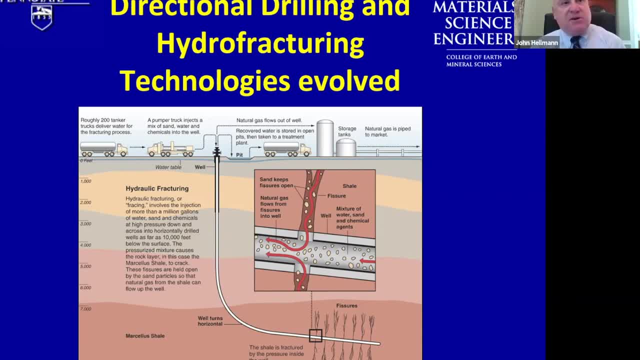 These deposits are on the order of 6,000 to 8,000 feet deep, And so this is a very long drill string that, once turned, can extend on the order of a couple miles. Those drill strings, or those drill bores, are then cased with steel, cemented with grout. 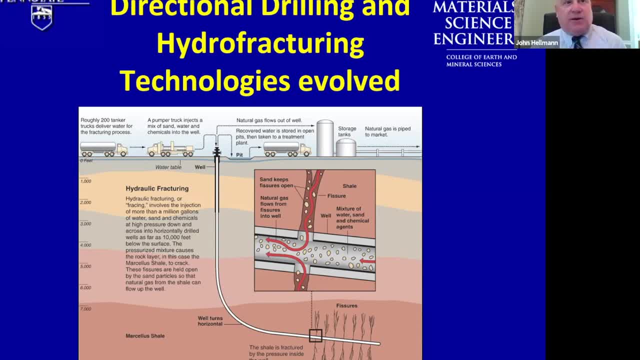 to the surrounding rock so that you have a relatively impermeable barrier and hermeticity to the surface so that you can avoid contaminating groundwater. You then subsequently introduce shape charges into the well bore And these shape charges are used to blast holes through the well bore. 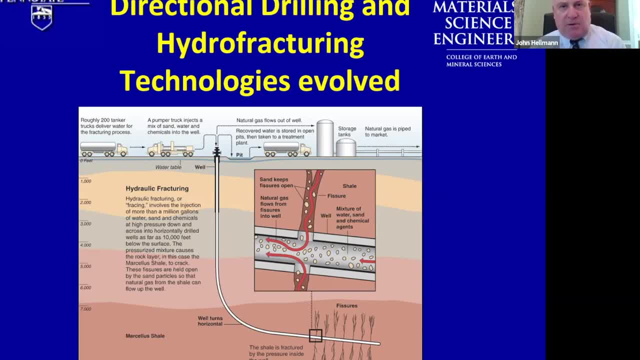 creating fractures in the surrounding shale. Those fractures in the surrounding shale are what release the natural gas from the shale to the well bore. But the intent is to increase the size and lengths of those fractures in the rock to be able to achieve more surface area. 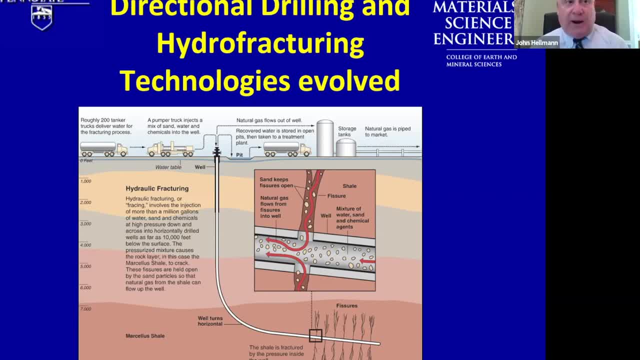 and retrieve more gas. Hence hydro fracturing is employed, where millions of gallons of water laced with ceramic particles, known as propants, are injected into the well bore. The well bore is then pressurized and these cracks that were created by the shape charges expand, grow. 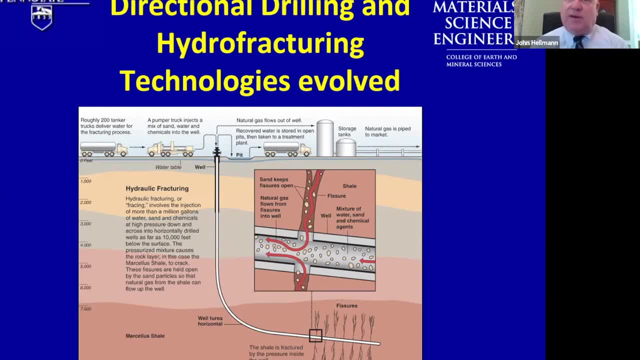 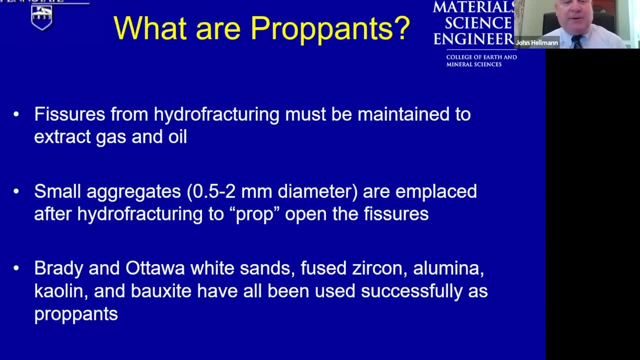 and are held open by the ceramic particles in the hydro fracturing mix, the propants. So the intent is that for a propant to perform well, they need to be sized in the range of about a half a millimeter to two millimeters in diameter. 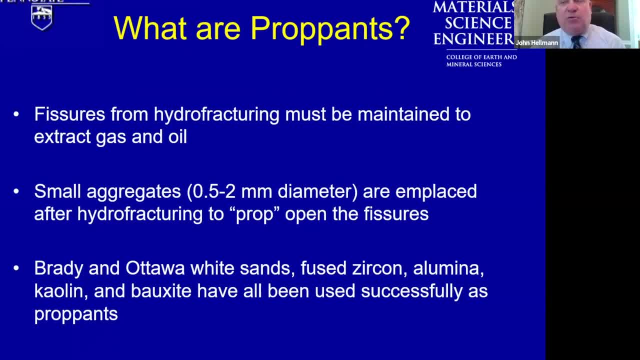 They need to be strong, easily transportable, robust in down bore chemical environments and available relatively inexpensively. That's an important characteristic, because something on the order of 1,500 to 3,000 tons of material are used to develop a single gas well. 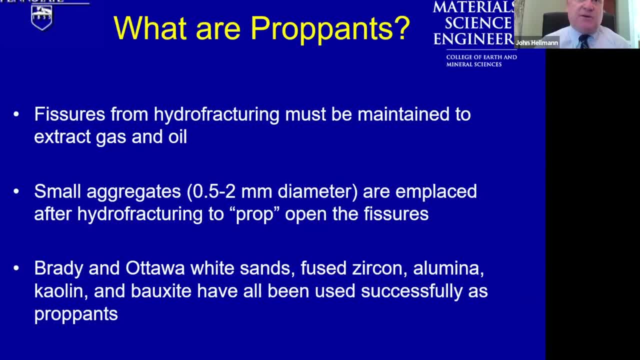 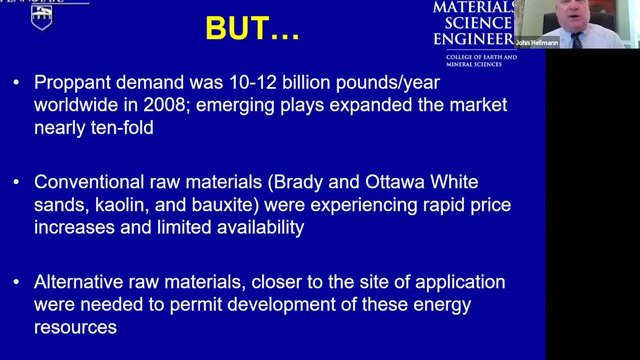 depending on the number of stages of fractures that were done during the shape charge blasting process. This is a large amount of material, So manufacturing capacity needs to be available and the costs need to be moderately low. But back about the time that these unconventional natural gas 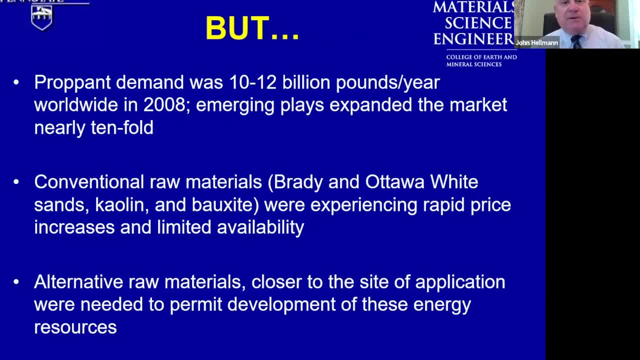 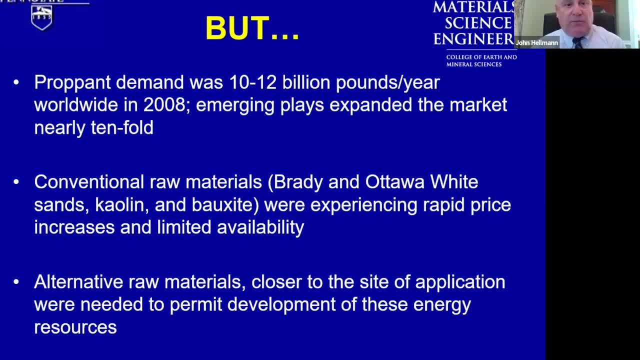 There was a rush on, for example, for the production of gas. There was a rush on, for example, for the production of gas And the demand for materials that could be used to prop hydro fractured gas wells And the conventional raw materials that were used as propants. 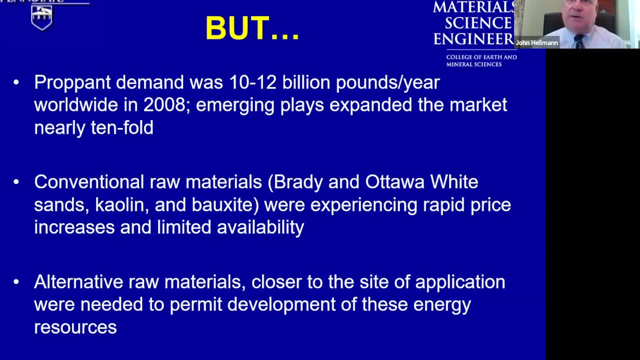 like the Brady and Ottawa white sands, kaolin and bauxite, sintered engineered propants and the like were experiencing very rapid price increases because of their limited availability and new demand. So alternative raw materials which are closer to the site of application, indigenous perhaps to the area, 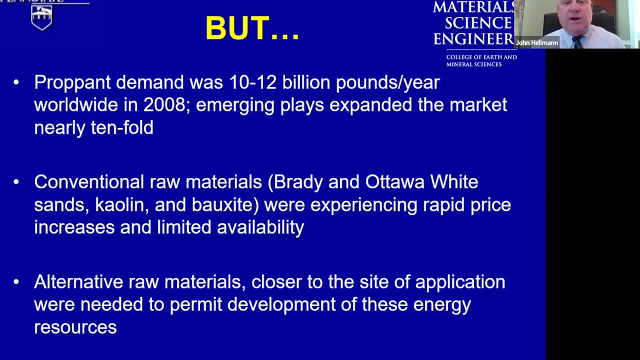 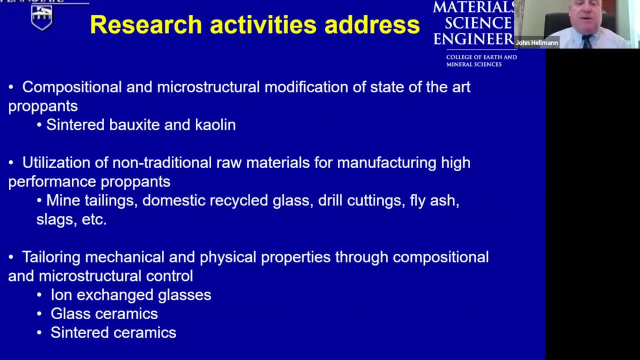 where natural gas development is occurring, were needed to permit development of these new energy resources. So the research activities we embarked upon were severalfold. The first was to take a look at the conventional commercial propant materials and manufacturing processes for those. 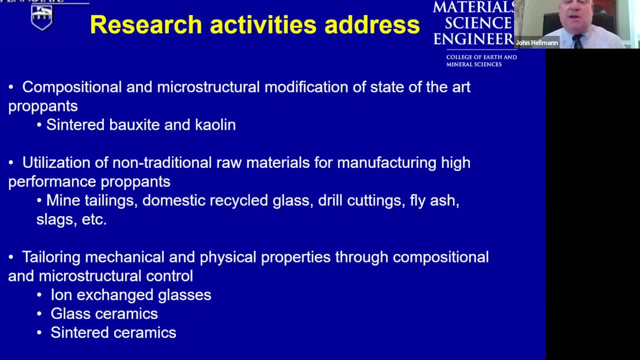 We were interested in understanding more about the compositional and microstructural models and modifications that would enable higher strength, lower cost of production and greater performance. We concentrated that work on the sintered bauxite and kaolin based propants that were commercially available. 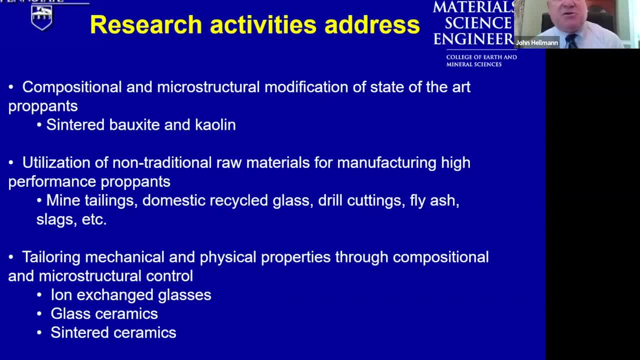 state-of-the-art materials, vintage 2002.. We also looked at nontraditional raw materials that are actually waste streams, byproducts of other industrial processes, For example, mine tailings, drill cuttings from drilling wells, domestic recycled glass, fly ash from coal combustion. 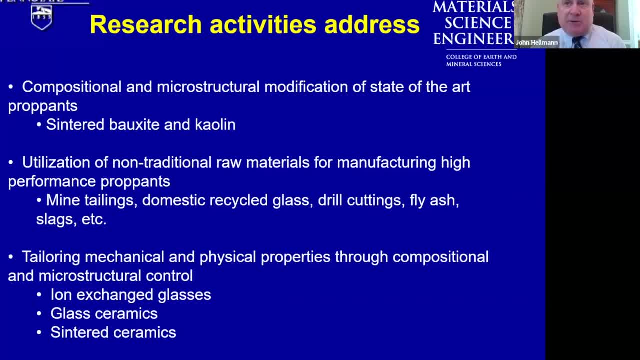 slags from metallurgical processes. These are typically materials that are put to landfill at significant cost and significant environmental impact, And we thought, if we could transform those into useful, value-added materials via good, well-informed ceramic processing technology, that we would have new value-added products. 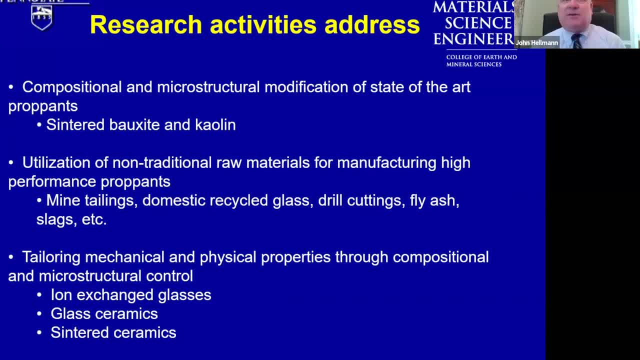 that, basically, are removed from the waste stream, giving significant economic and environmental benefits. The whole thrust in this work was to tailor the mechanical and physical properties of the materials through compositional and microstructural control, And we practiced this work in several different families. 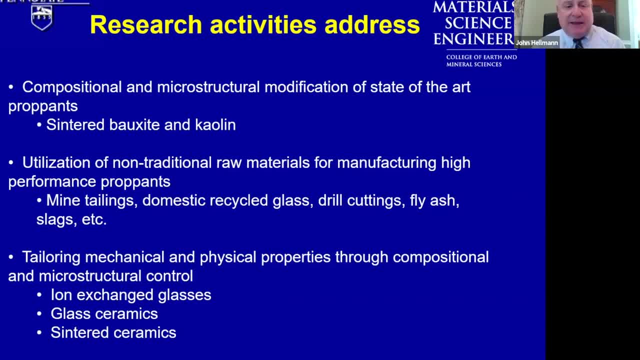 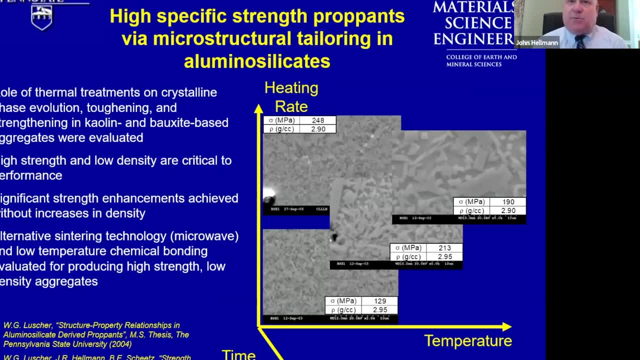 of materials- ion exchange glasses, glass ceramics and centered ceramics- And I'll tell you a bit about all of these. In the first case, where we wanted to examine what processing modifications could be done to enable us to manufacture propants cheaper and with a lower environmental impact, 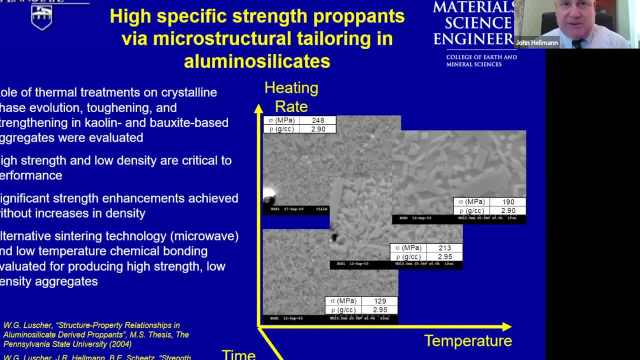 we practiced this on bauxite and kaolin-based propants. These were commercial materials where we accepted and expanded the range of centering temperatures, centering times and, interestingly, the heating rate to get to the centering temperatures. The heating rate is an important characteristic. 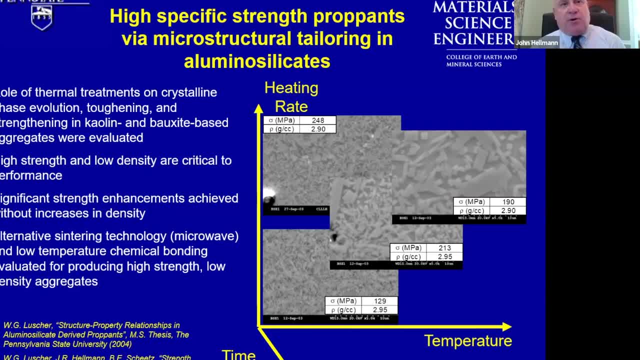 because these materials are centered in large rotary kilns, much like a cement clinker manufacturing process, And therefore not only the temperature that you go to but the residence time of the material during the centering process has an impact on the amount of hydrocarbons. 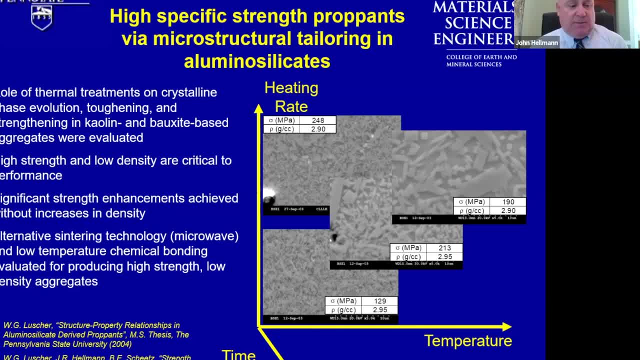 that you use as the fuel to heat the process, as well as the CO2 that's generated during the process. So lower centering temperatures and shorter centering times, which could be achievable by higher heating rates, are good things to consider, provided the mechanical 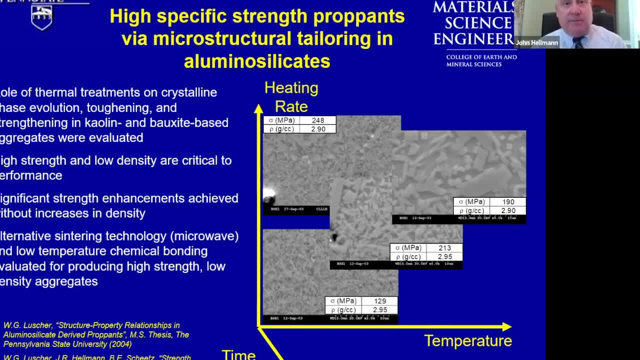 thermal and physical properties of the resulting propant is not modifiable. So we were able to demonstrate, in the case of bauxite and kaolin ores, that we could center the materials at substantially lower temperatures by manipulating heating rates, going to higher heating rates. 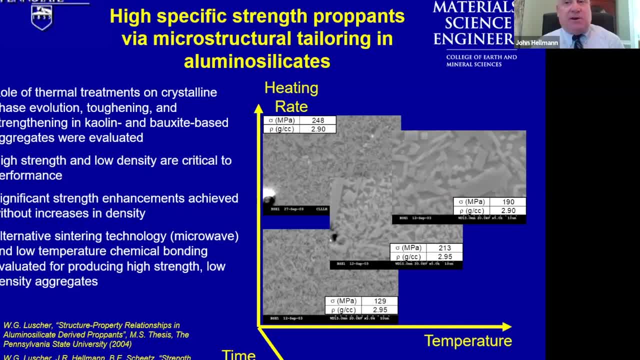 and achieving fine microstructures, fine grain size microstructures, appropriate crystalline phase assemblages and specific gravities to yield high compressive strengths. This was good news at the time. Industrial processes were able to be modified, Economic benefits and environmental benefits were achieved. 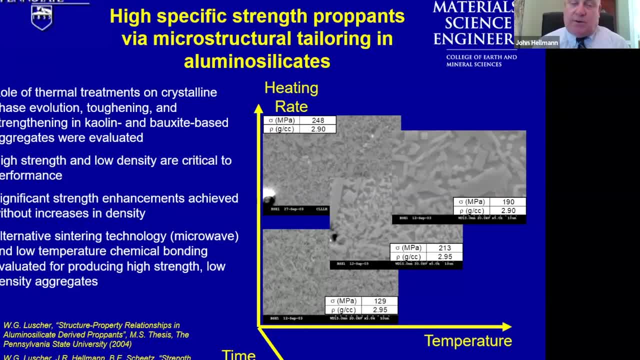 Well, in the course of doing this work, we thought: what could we do to improve the centering process even further, to permit even lower centering temperatures and perhaps even finer microstructural evolution? And so we embarked upon trying to understand what could we do to improve the centering process. 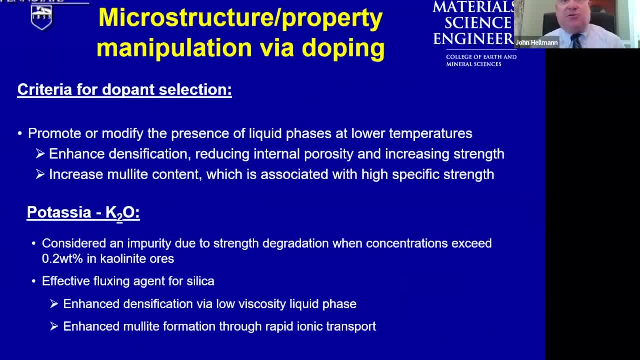 in a way that would allow us to be able to reduce the viscosity of the liquid phase during the centering process, increase ionic transport and indeed also take advantage of transient liquid phase centering mechanisms to yield high degrees of densification, appropriate phase evolution. 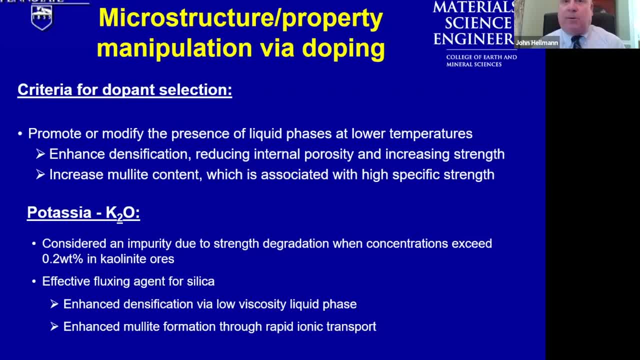 and high strength propants. So we looked at a number of different ways to improve the centering process. We looked at systems in which potassium oxide and iron oxide were deliberately doped into bauxites and kaolins at levels higher than what were considered to be. 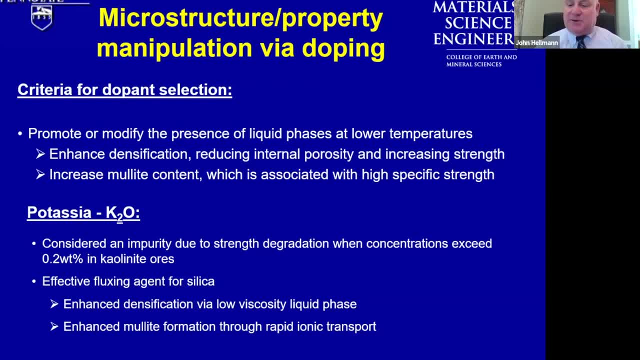 excessively high impurity levels by the prop and industry at the time. This was a hard sell in the beginning. Why use more impure ores to make these materials than what was typically used in the past? Well, the driver on that was also economic. 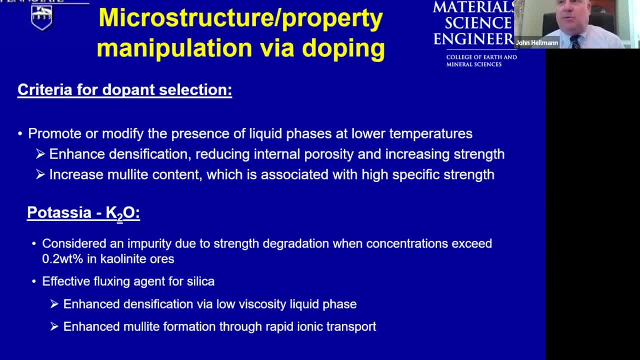 Well, the driver on that was also economic. Well, the driver on that was also economic Because the ores that were available outside of our domestic confines of the continental United States had higher levels of potassium and higher levels of iron oxide, And in the past it did not result in. 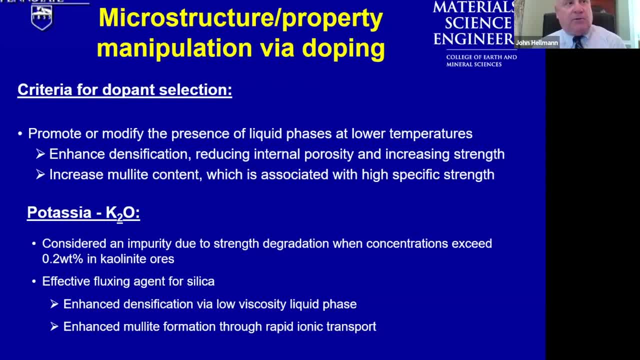 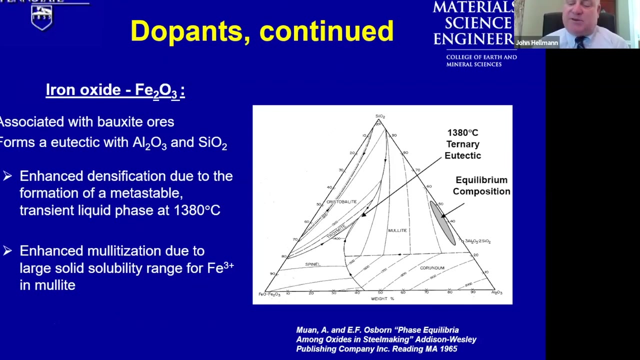 or allow production of prop and particles of sufficient mechanical properties for use in the oil and gas industry. So we embarked upon a series of experiments in which we dramatically expanded the level of dopant concentrations outside of the common impurity levels. We exploited transient liquid phase sintering. 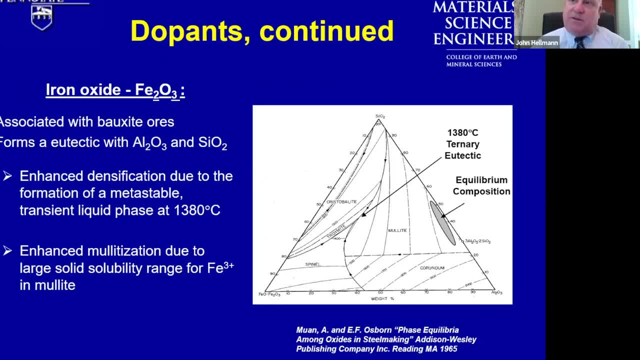 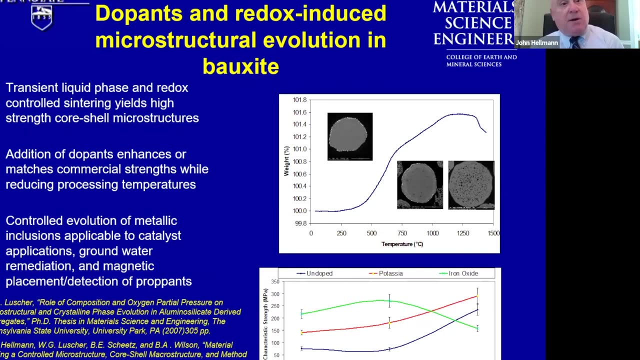 to achieve high levels and rapid densification, at the same time achieving requisite crystalline phase assemblages to achieve high strength. And some interesting things cropped up. We were able to densify the materials at a couple hundred degrees lower than normal. We were able to densify the materials at a couple hundred degrees lower than normal. 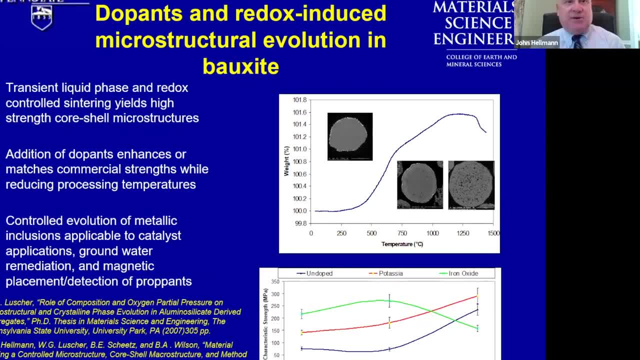 We were able to densify the materials at a couple hundred degrees lower than normal, Than what was traditionally being used in the prop industry to get full density and high strength In the prop industry. to get full density and high strength, Strengths commensurate with the very best. 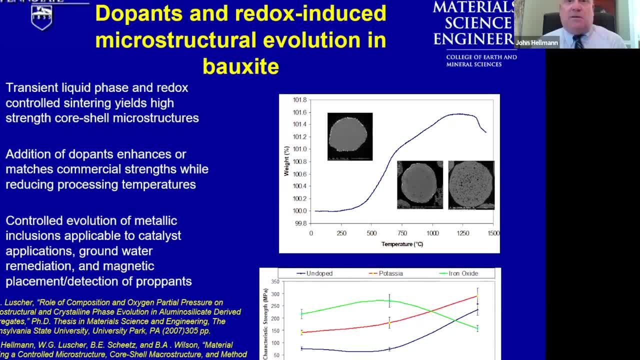 commercial state of the art materials. The interesting thing that we also saw is that in these dense particles, at the conclusion of the sintering they were oftentimes decorated with metallic iron, which was a bit surprising to us, because the sintering processes 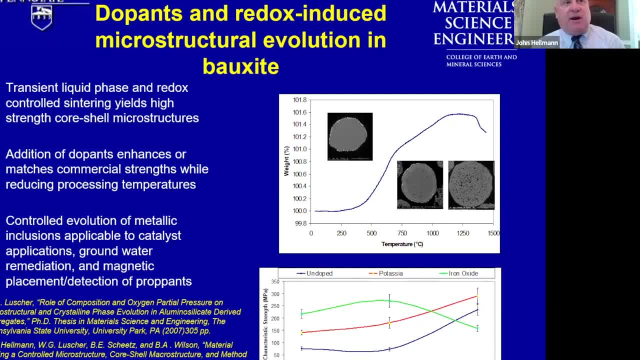 are done in a combustion environment, environment where the combustion environment is relatively oxidizing. We didn't expect to see metallic iron. We redid the experiment several times because we didn't believe the results, And indeed every time the same result cropped up. So we dug further into the literature. 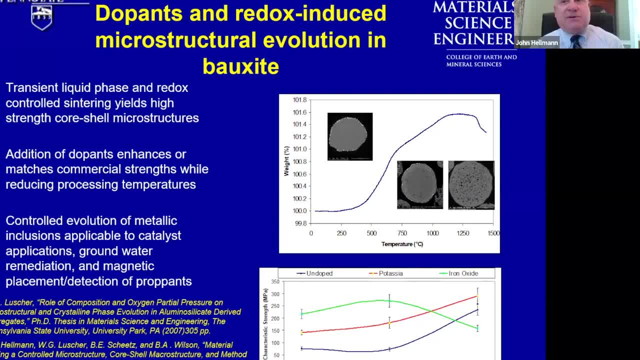 literature going back to the 50s from the refractories industry and understanding the interactions between fireclay refractories and bauxite-based refractories with molten iron, steel and slags, And what we found is that the occurrence of these metallic iron 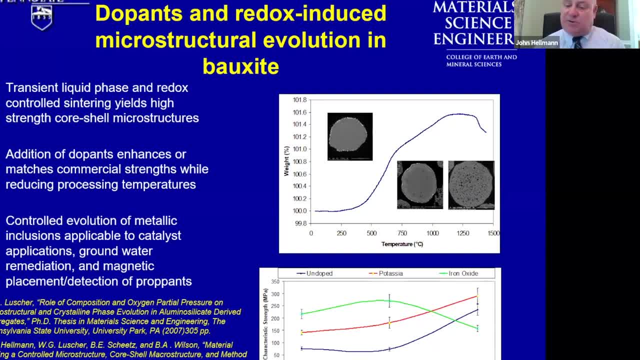 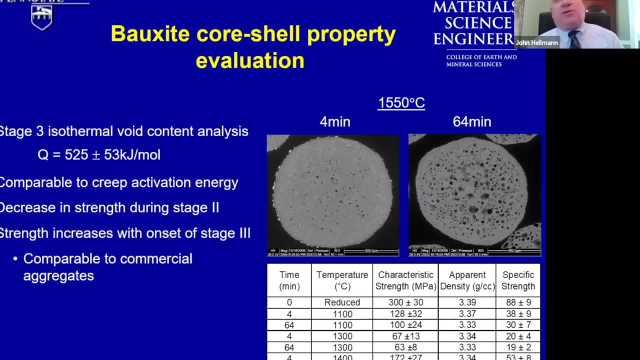 decorations on the surfaces of our particles was entirely expected if we understood more about the oxygen partial pressures through the course of the processing cycle, And so we thought this would be an opportunity. Could we exploit those iron decorations to re-react with the material in subsequent phases of the centering cycle to form a dense 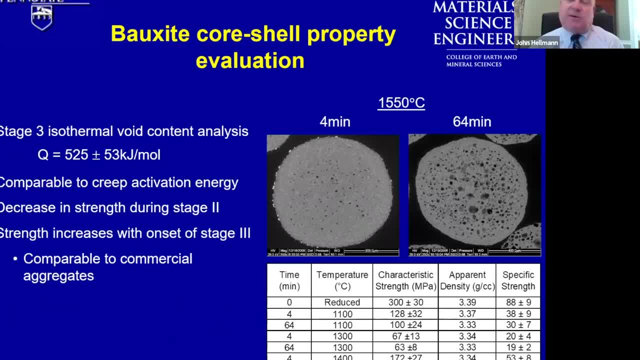 outer core and potentially a porous or a dense outer layer shell and a potentially porous inner core. And indeed we were able to do that. And here's what we saw If we started with a fully dense, fully densified prop and particle achieved by our centering. 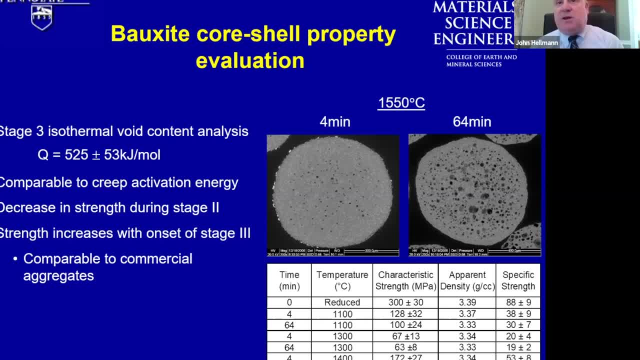 process I just showed you and then subsequently reheated it in a controlled oxygen partial pressure. we could evolve porosity in the interior of the particle while maintaining a dense outer shell. We studied the kinetics of that process and found that the activation energy of the pore evolution was on the order of 500 kilojoules per mole. 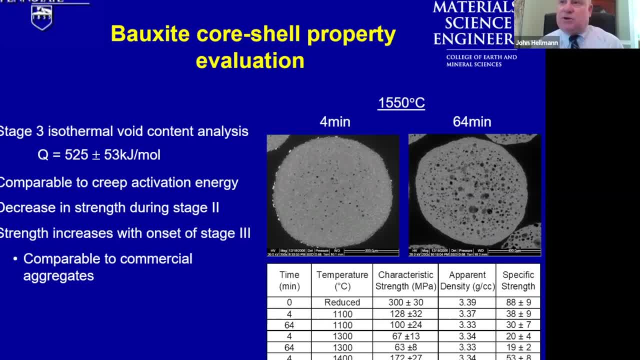 Which is comparable to the creep activation energy of aluminosilicates of this composition. This is an interesting result because it supported our hypothesis that the evolution of this porosity in an already dense ceramic was the result of evolution of oxygen blowing bubbles. 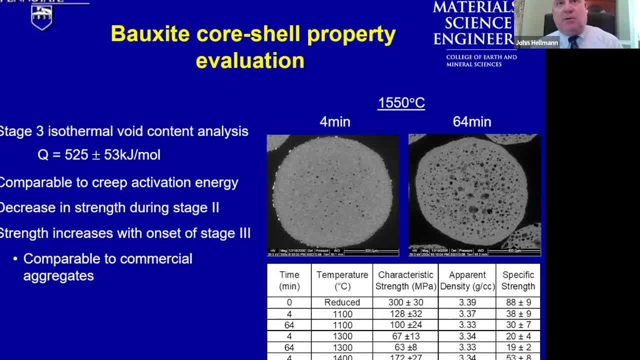 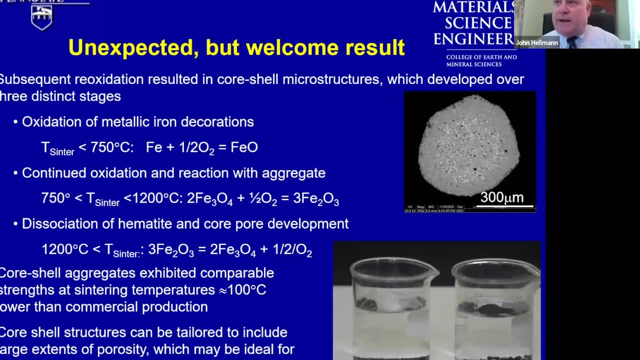 if you will, in the interior of the ceramic particle when you process the material in a controlled oxygen partial pressure. This was a borne out in subsequent studies and it allowed us to manufacture propants with what we term the core shell microstructure, Where we take a ceramic particle or propant, center it to full density and then de-densify it while maintaining a dense outer shell. 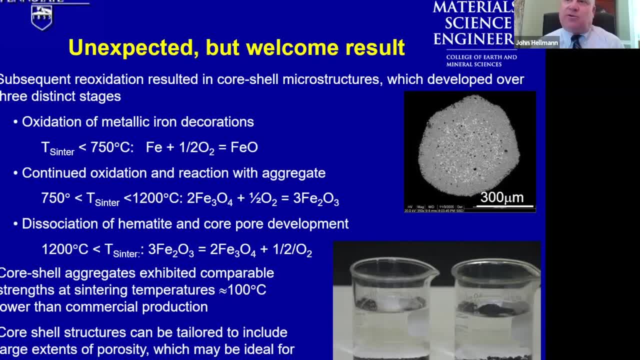 This yields a hermetic particle with controlled specific gravity to the point where you can make a neutrally buoyant ceramic propant, a propant that floats in water, Which has significant environmental benefits as well, as well as economic benefits, because most hydro fracturing liquids are laced with different chemical species to promote the 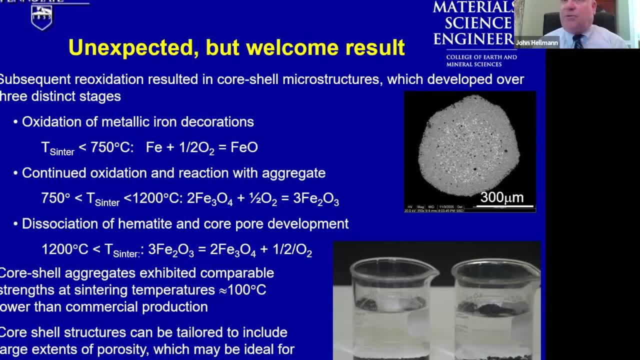 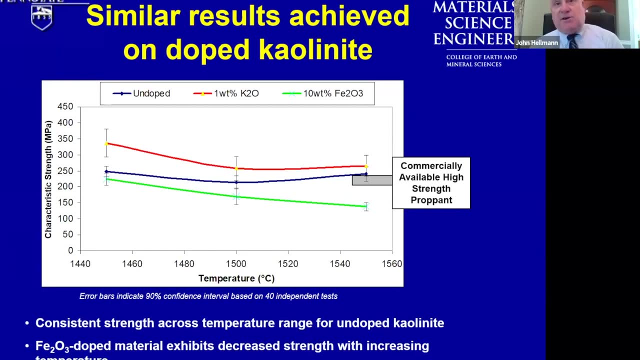 suspension of the propant particles in the hydro fracturing fluid during the injection process. A neutrally buoyant particle will require fewer of those chemicals- a significant environmental impact improvement. So we're back with the next slide. Next slide: We'll be back in about an hour. 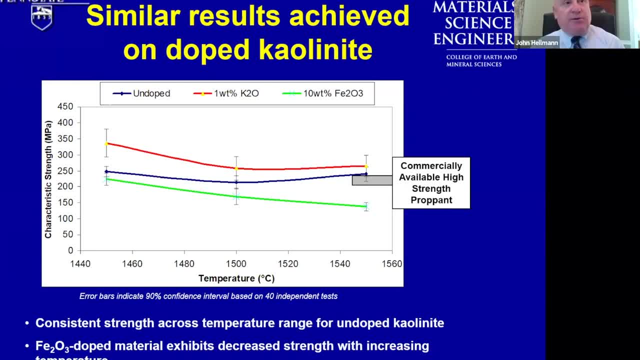 Similar results were achieved in the doped kaolinites. We were able to center these at substantially lower temperatures, and we were also able to achieve the malted milk ball or core shell microstructures in these materials by exploiting the use of the iron oxide doping. 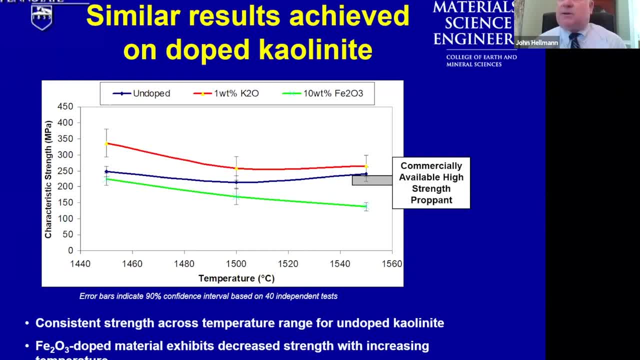 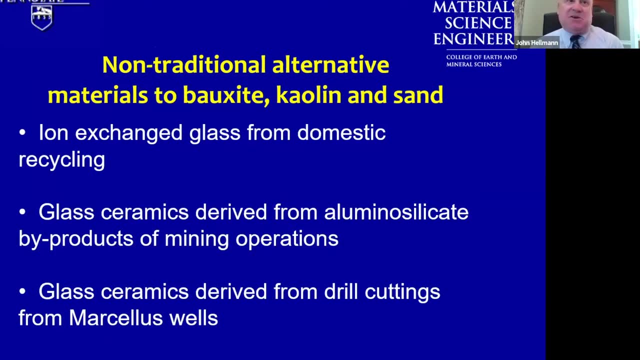 While we patented that work, that work was subsequently licensed. it's being exploited in the manufacturing of controlled specific gravity high-strength propans right now, which are being used around the world. We shifted our attention, or continued our attention, into other materials. 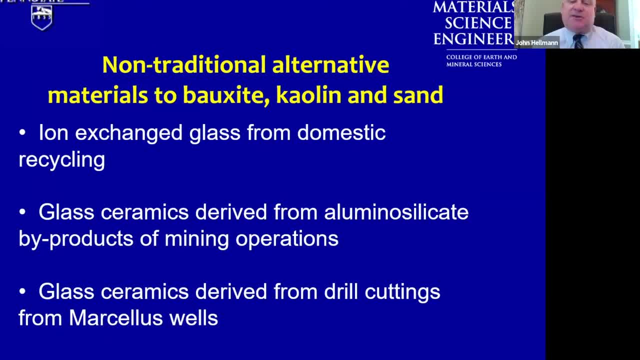 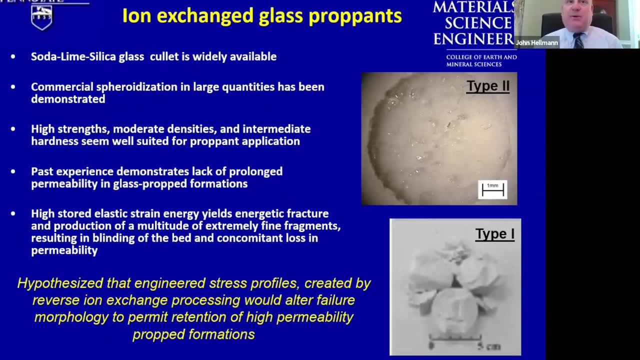 I'm going to tell you a bit about each of these: ion exchange glass for use as propans, glass ceramics derived from mine tailings and glass ceramics derived from drill cuttings from wells. Let me start with the ion exchange glasses. Glasses have been considered for use as propans for decades. 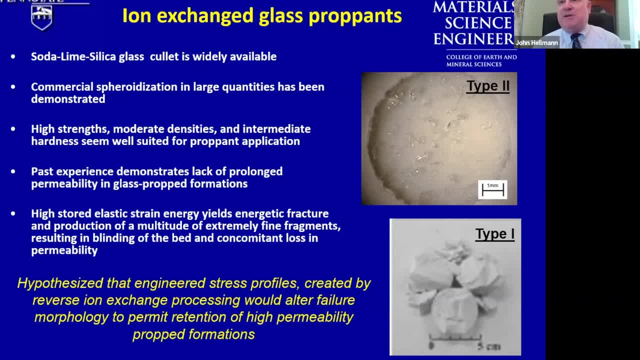 Glass particles that are highly spherical can be manufactured in very high-strength form using flame spheritization processing. They're readily available, and available in the kinds of quantities that would be commensurate with use as hydrofracturing additions. However, they don't work. 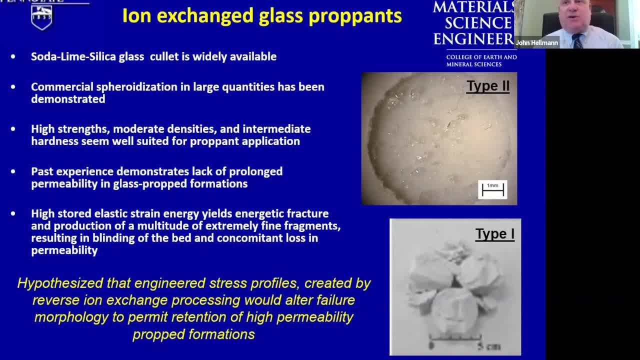 And they don't work because they're such high-strength. What happens to a glass particle when used as a propan is that when the pressure of the overburden, the closure stresses in the well is significantly high, on the order of 6,000. 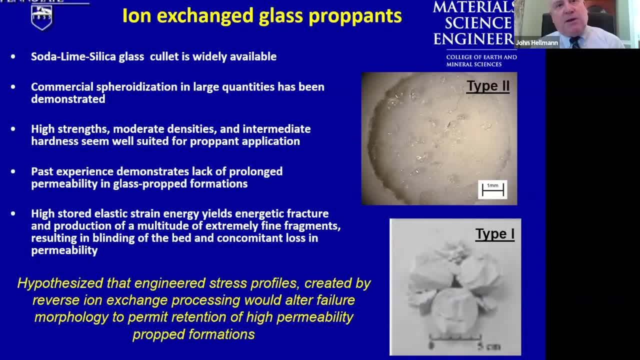 psi or so these beads fail. And when they fail they fail into very, very small particulates. These small particulates are the result of the high stored elastic strain energy. at failure, Those small particulates in turn blind the interspaces in the remainder of the prop particle bed. 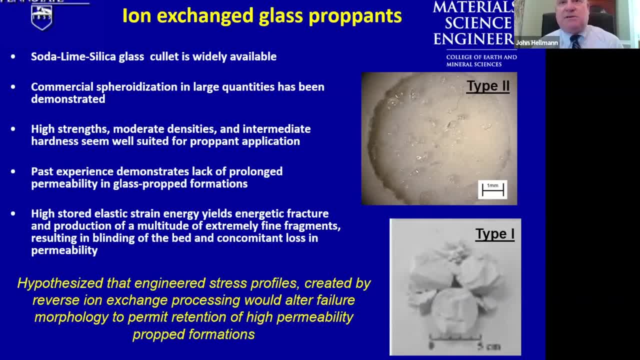 And, as a result, the permeability of the bed is decreased, thereby decreasing the production rate of the well. So glass is not used as propans. That's unfortunate, because domestic glass recycling streams are enormous in the United States And they're ubiquitous. 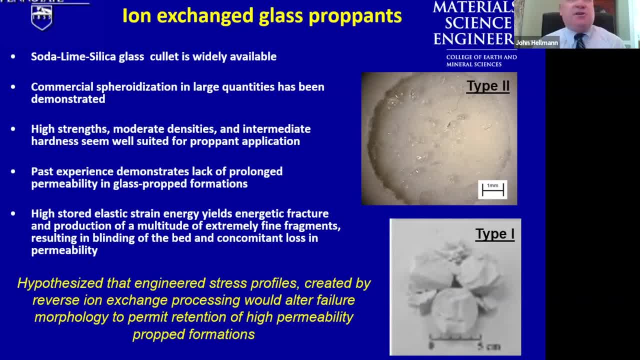 They're all over the place. They're indigenous to areas where natural gas exploration and development is occurring and could be readily exploited if they could be made to work properly. So we hypothesized that we could modify the behavior of glass particles by engineering stress profiles in the propan particles in such a way to make them fail into large chunks. 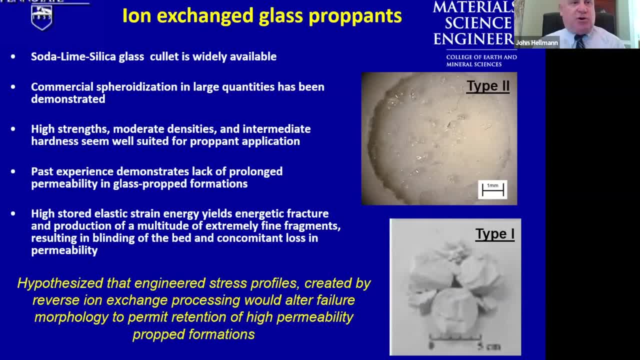 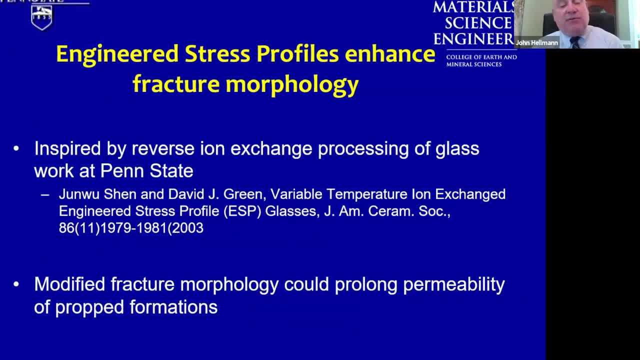 instead of fine particulates, and those large chunks would continue to prop. This work was inspired by things that were being done by my colleagues Dave Green and Jun Wu Shen at Penn State at the time on engineered stress profiles in reverse ion exchange glasses. We thought that we could apply the knowledge that 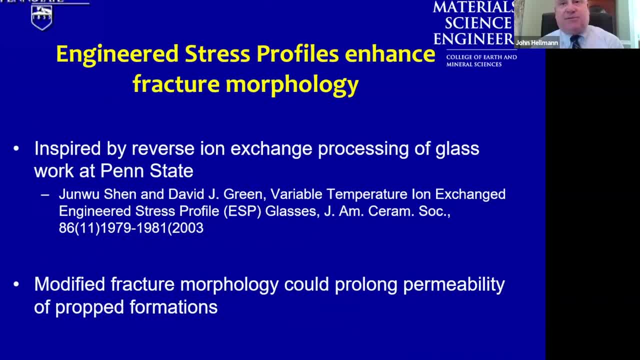 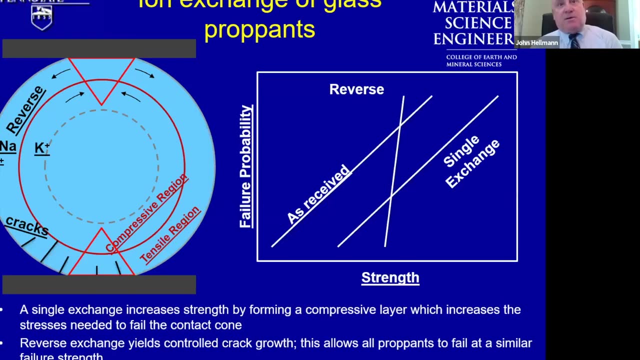 they were generating there, to the development of a new class of propants based on glasses, which would perform in an admirable way. This would be done by modifying the fracture morphology and hence prolonging the permeability of prop formations. This cartoon here shows you what the 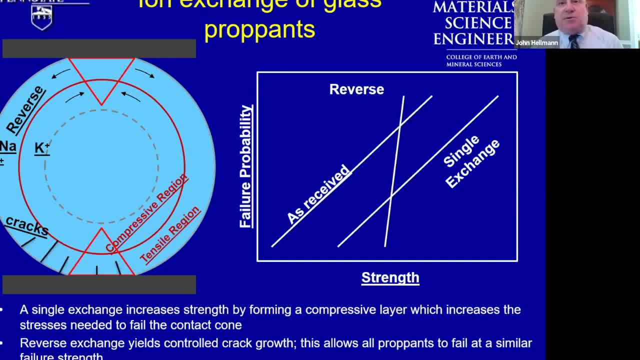 concept would be, That is, we would start with a prop and particle manufactured from glass, in which we remove some sodium, replace it with potassium using a molten salt ion exchange process and then, using a reverse ion exchange process, put some of the sodium back. What this would result in is a tensile. 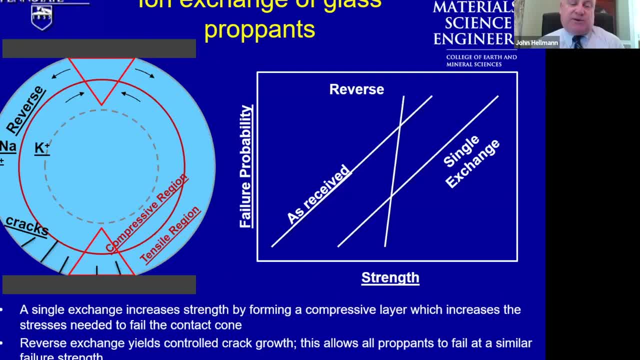 region at the surface and an embedded compressive stress field in the prop and particle, which would have a couple of benefits. The first is the inherent flaws at the surfaces of the glass. particles would all grow to a finite, uniform length. They would arrest at the boundary between: 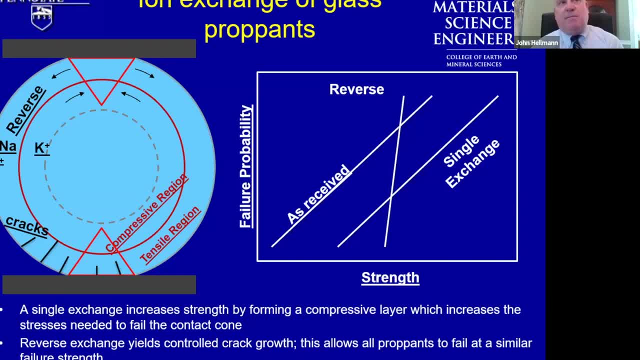 the tensile and the compressive stress field. The second is the compressive stress field would yield high uniformity and strength and give degree of granularity to the groups beyond the tensile and textured spaces. Tada a very high akanum both in a protective and least. 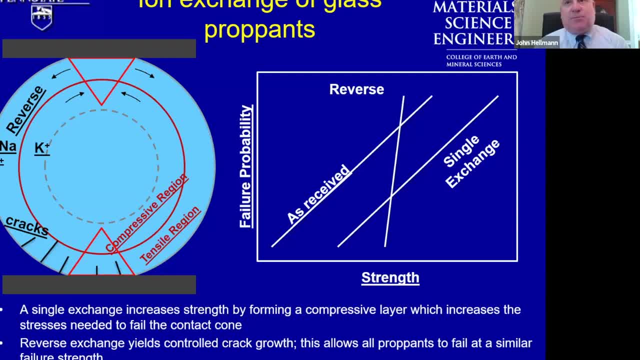 orders. hadi clicking block has an alternative solid fiber which will allow for more condniejsisce to the FeAsur in the proactive NOирt beam. The third contribution went into high uniformity, przedstawlente, significant strength, particularly in the пожалуйстаiling of皆さん ing a highly reliable chaque particle of tensile stress field. 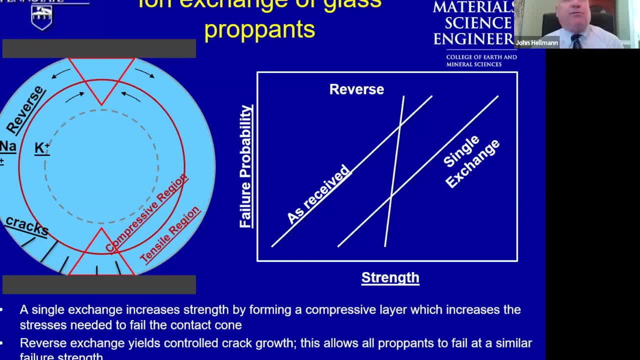 Yielding a particularly Koh-i-Met- it i heighly- conternable strength. potentially stronger as well. Secondly, the compressive-wide stress profile 챡 mpe, densaile stress profile and transition to the tensile stress field. transmissionostreicalp scle ia. 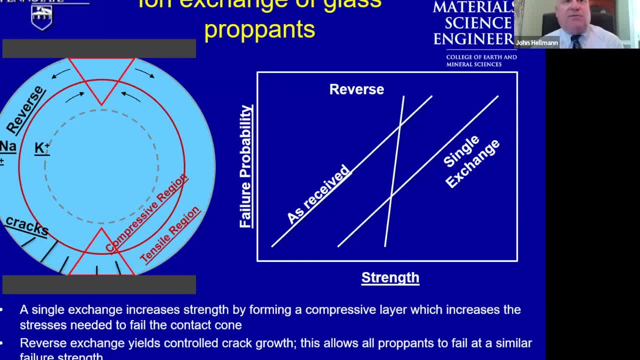 might contribute to an onion-skin failure-type morfolgreide, which the outer layers of the particle would Steroe, consecure a fquelesающelouましょう compressive loading, leaving behind a large inner core which could still prop, and that was verified. 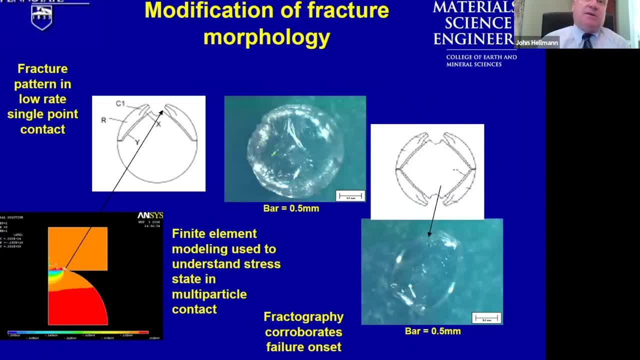 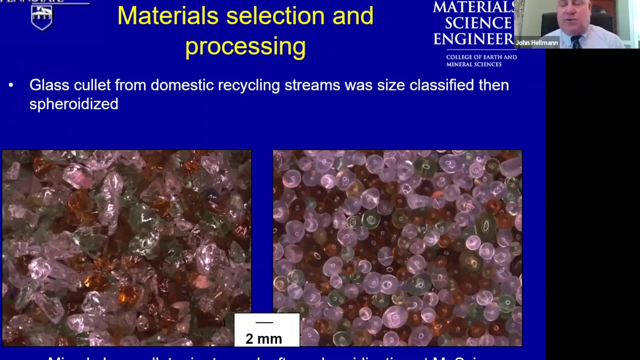 using finite element analysis on union exchange glasses that this failure process could indeed be stimulated. these are from finite element modeling of compressive failure of beads of glass particles using an api 60 test methodology and we thought that we'd be able to accentuate that through the use of a reverse ion exchange process. so we procured glass cullet from 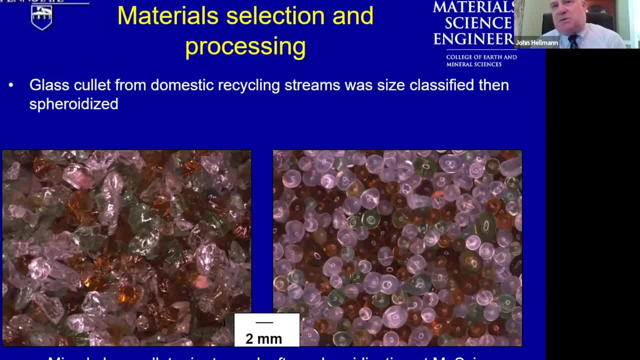 the domestic recycling glass industry. this is glasses of a variety of colors, all from your beverage containers and the like. so you'll see green, you'll see brown, you'll see clear, occasionally even blue. we worked with moci then to spheridize these using their flame spheridization processes. 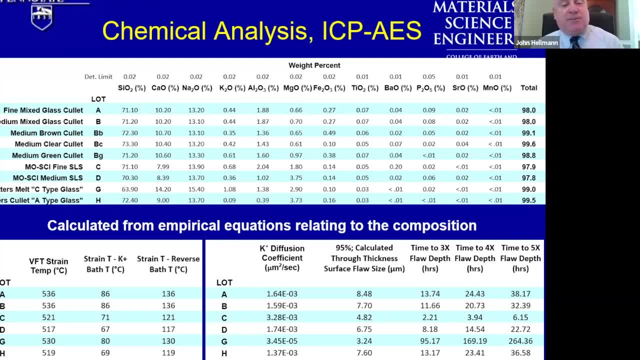 we characterized their chemistries, which was an important thing because we needed to know how to ion exchange the materials to different levels of starting flaw depths. so we used this information to calculate things like strain temperatures and temp and temperature time behavior necessary to embed a compressive stress field at a depth of one, three, four and five times the initial starting flaw depths. 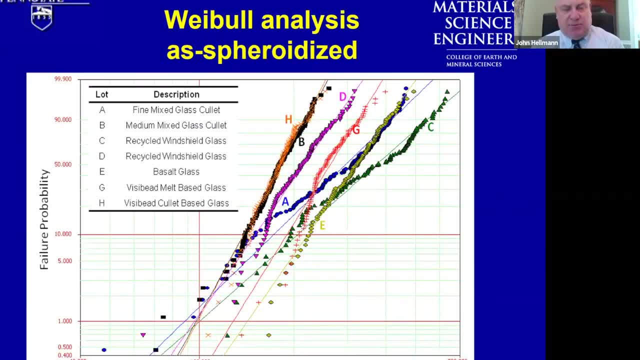 we used weibull analysis to characterize the strength distributions. these are weibull distributions based on hundreds of individual fractures in diametral compression of a variety of different glass bead materials. we use this methodology throughout because it enabled us, number one, to understand the characteristic strength. 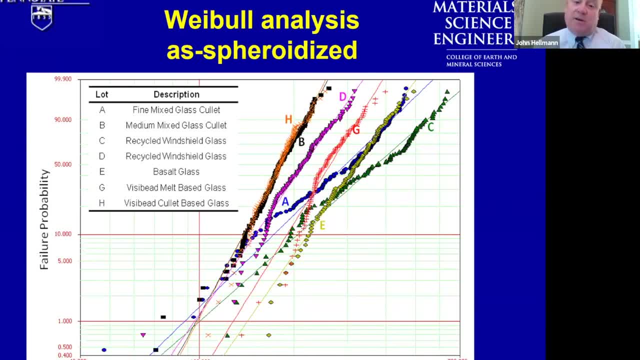 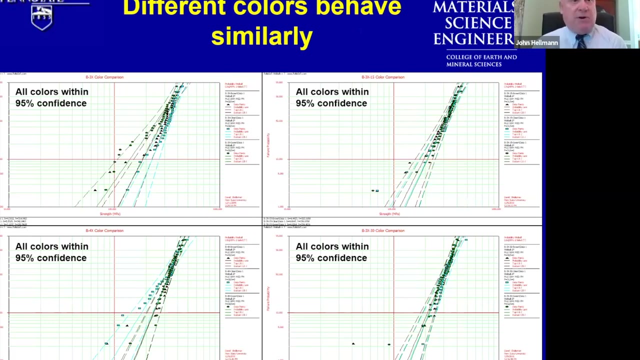 number two understand strength, uniformity. and number three: we could then use that data to calculate the onset of failure and strength of any bead of comparable composition and treatment but of a different size or under a different loading characteristic. We found the colors behaved similarly. There was no difference. We don't need to separate. 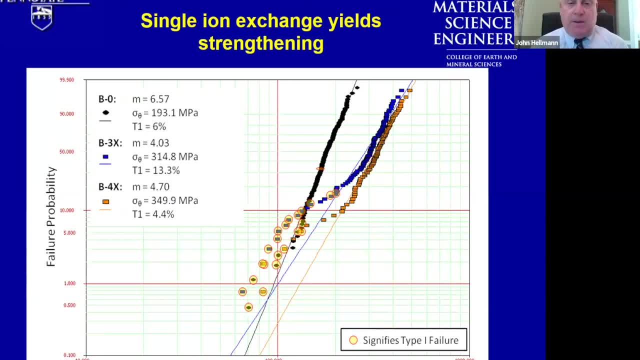 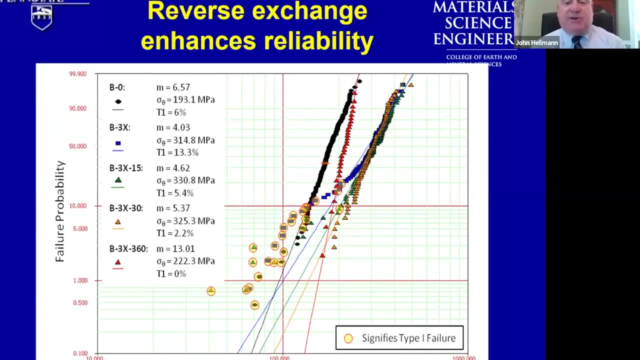 the different colored glasses for this application and that single ion exchange yielded strengthening, as was expected, and reverse ion exchange enhanced the reliability also, as we originally hypothesized and has been seen on other types of glass articles. Furthermore, longer reverse ion exchange types. 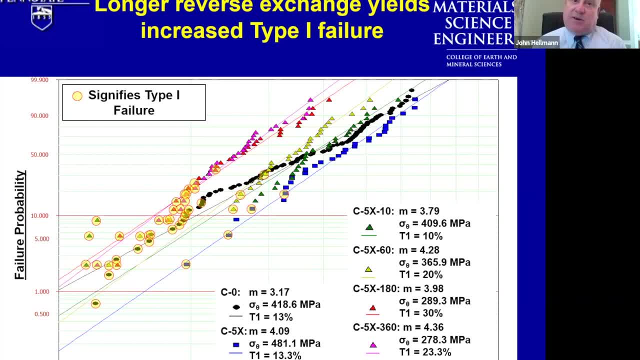 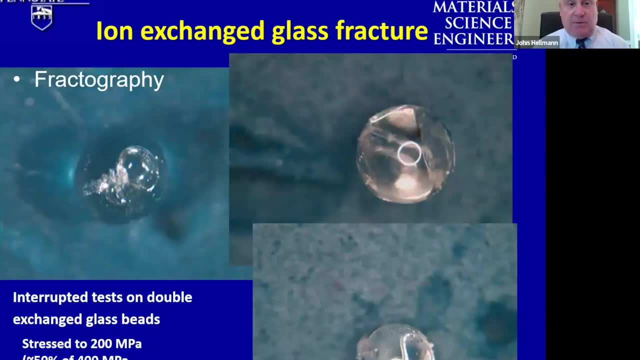 exchange processes yielded increased occurrence of type I failure. Type I failure is the failure of the propane particle into large chunks, not fine particulates. Type I failure is desirable for their application as products. We verified that this failure process was indeed occurring using interrupted load tests. This particular bead was stressed to on the order of about. 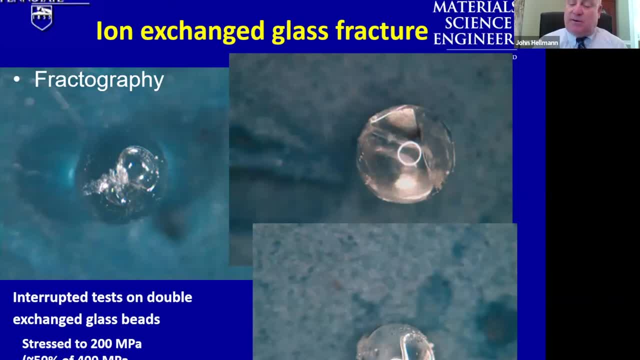 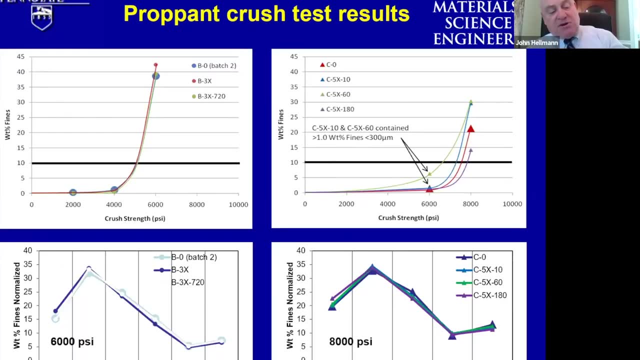 half Of its characteristic strength and then fractography was performed. We also employed American Petroleum Institute standard test methodologies to understand how these propane particles before and after ion exchange performed in crush tests. Now, a crush test from the American Petroleum Institute entails taking an assemblage of beads. 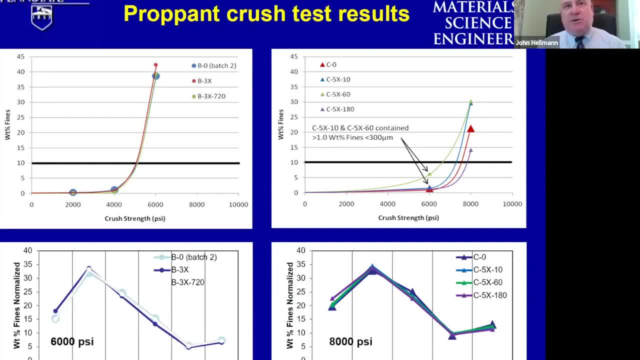 in a dye applying a uniaxial load to different levels, sieving the materials in-between loads. When 10% of the materials is produced as fines, that is considered the crush strength. Pretty empirical, but it is used widely by the industry. What we were able to demonstrate was 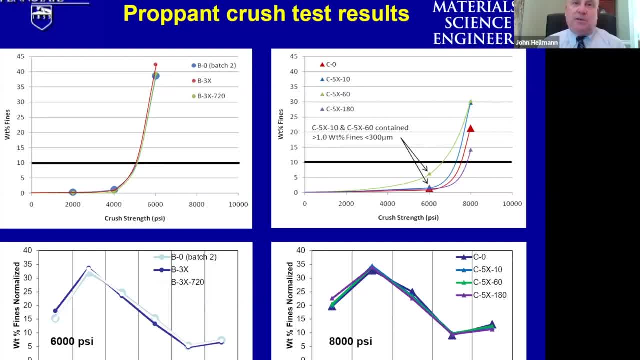 that our ion exchange glasses outperformed things like sand and a few other materials that were available for use as propane in large tonnage quantities. These materials perform well to 8,000 PSI, which is good news. Those are pressures that are consistent with their use. 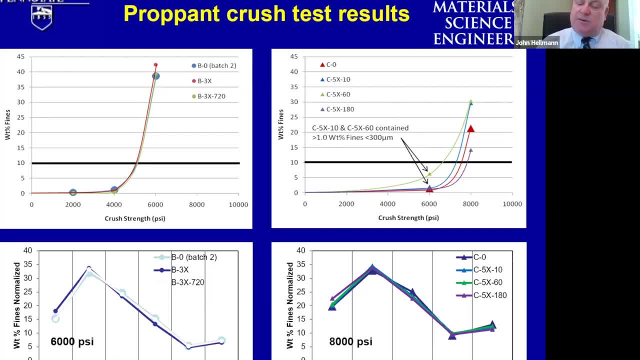 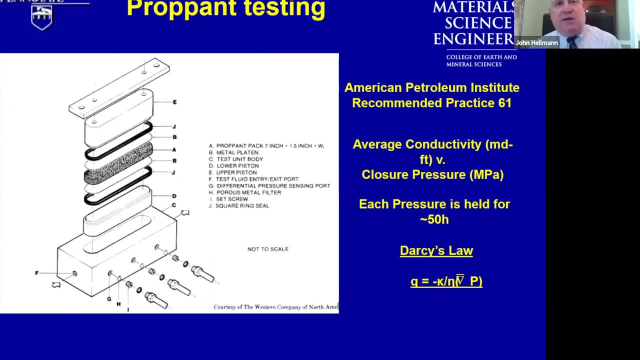 in both the Utica and Marcella shales, and perhaps even out in the Bakken. We then moved on to understanding how these materials behave with respect to permeability. Liquid and gas permeability is measured using an American Petroleum Institute 61 standard test That's now known as the ISO 13503-2 test, in which an assemblage of particles 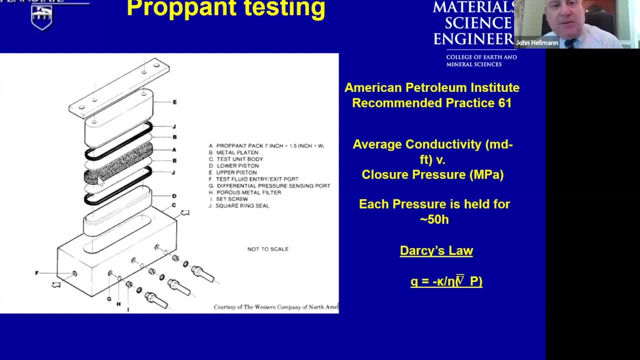 is constrained in a steel die and a uniaxial load is applied via platens. A liquid solution of KCl in water, potassium chloride in water, is passed through the particle bed and pressure drops are measured using potassium chloride. Using this, we can calculate, and using Darcy's law, the permeability of that packed particle bed. 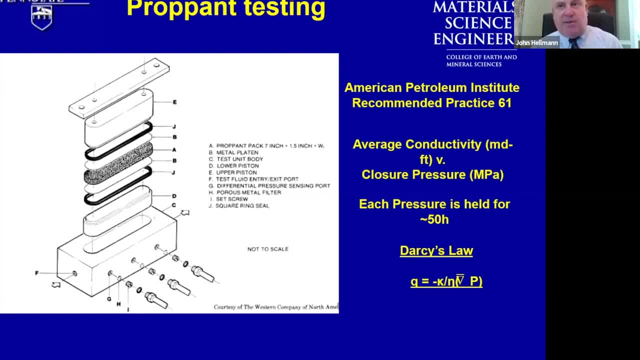 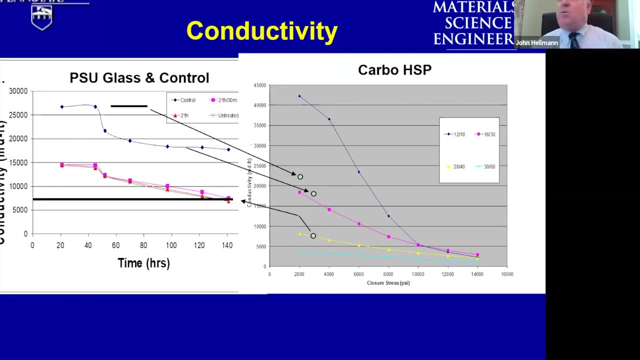 as a function of the uniaxial load And that will tell us how useful that particular prop and particle type is for use in stimulating oil and gas wells. These are some of the results that we achieved and basically what we found is that the ion 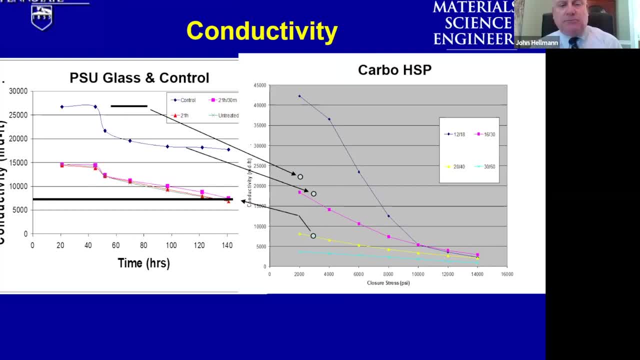 exchange was not as good as it was in the past. The ion exchange glasses perform admirably well, so do some of our other materials relative to high-strength ceramic propents manufactured in industry, and that they're performing this way without the application of coatings, which is a common practice for. 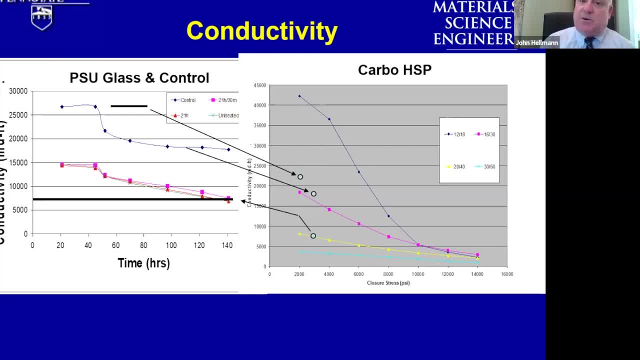 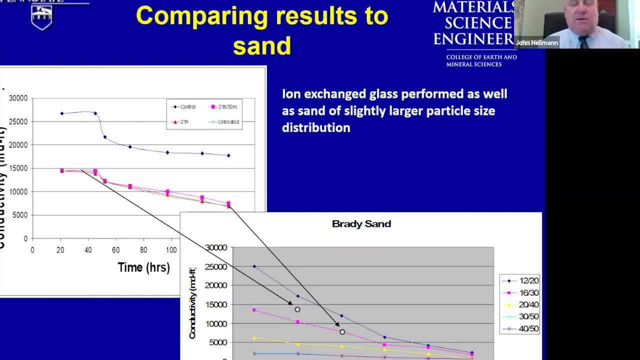 high-performance propents in the industry. Coatings are typically phenolic resins and they're expensive to apply. If you don't need them, don't use them. These are some of the results that we achieved and basically what we found is that the ion 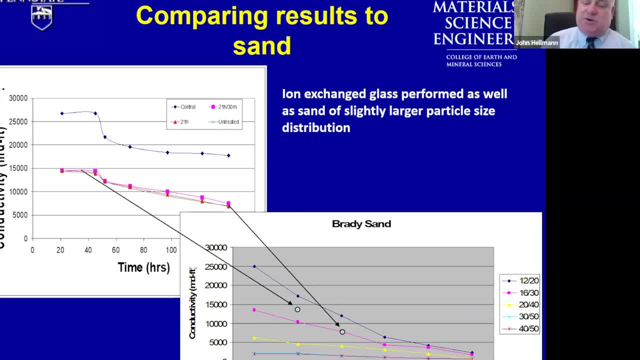 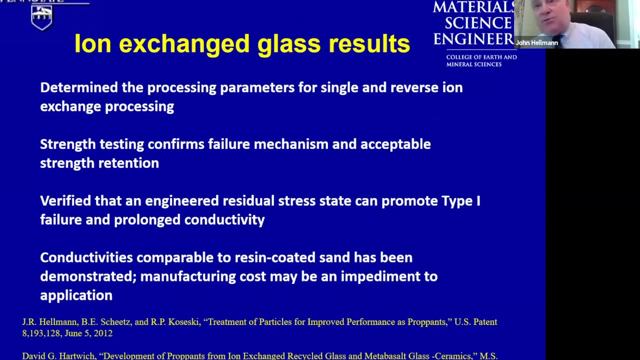 exchange glasses perform admirably well, so these materials outperform sands, which is good news. We can use these to prop to deeper depths for longer periods of time. So these were all great results. The ion exchange processing looked very promising. The strength testing confirmed the failure mechanisms we proposed and we had acceptable. 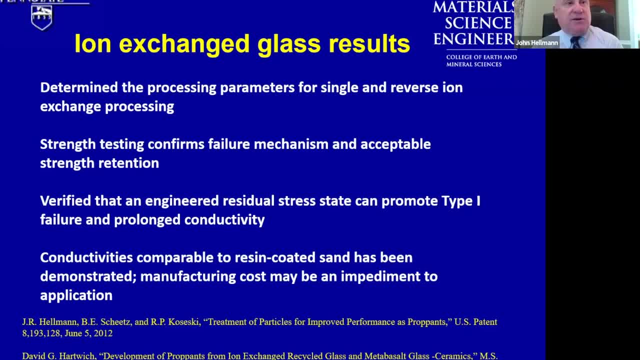 strength retention. We verified, using the engineered stress state, finite element analyses and the like, that we can promote type 1 failure and prolonged conductivity impact beds. However, these are ion exchange glasses. They need to be manufactured in thousand tonnage quantities. That's a large amount of material and it's an engineering challenge to ion exchange. 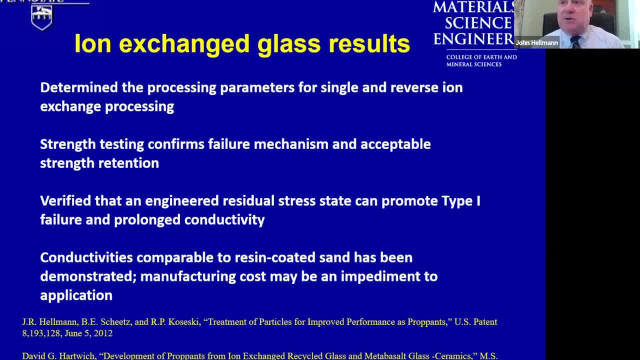 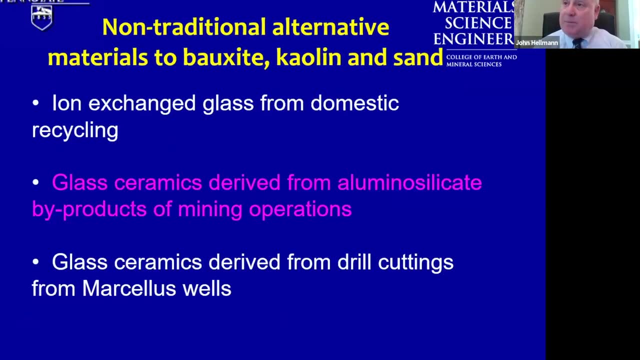 and reverse ion exchange that quantity of materials and that might impact the economics of the process. At the same time we were working on other materials, so we segued into those that paid more attention. Glass ceramics derived from aluminosilicate byproducts of mining. 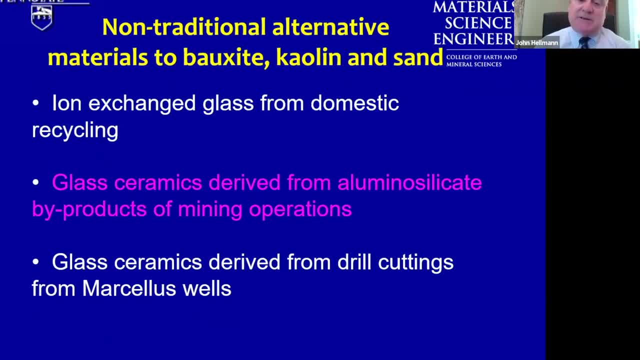 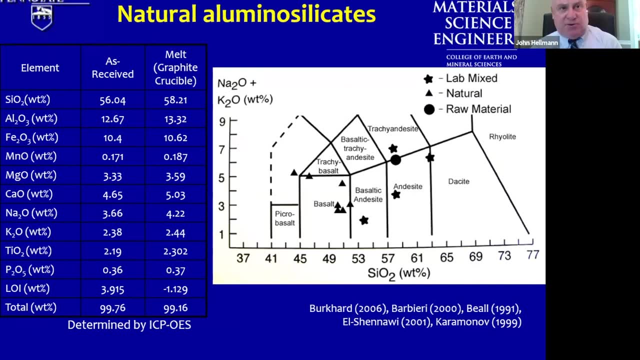 operations is where we directed our attention. next, These are materials that are derived from what are essentially basalt compositions. These basalt compositions started as volcanic glasses, which subsequently then crystallized over the eons to form the basalts we're all aware of. 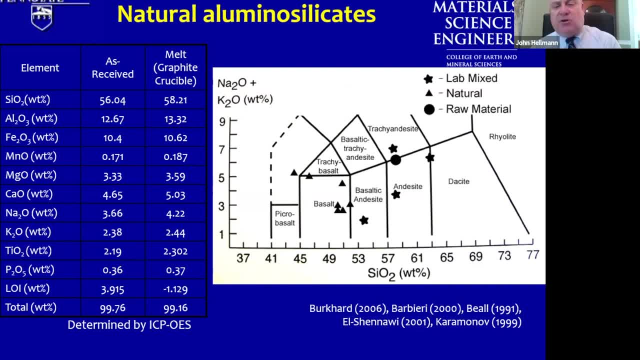 So things like andesite, rhyolite and basalt are the areas that we worked with. Why? Because these materials are available in massive quantities as an industrial byproduct of the roofing granule industry. Materials like basalt, andesite and rhyolite are routinely 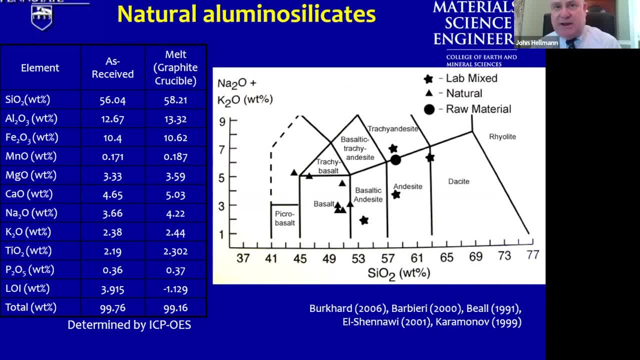 machined, crushed, sized to a particular size fraction and then used as granules on asphalt shingles used in the building industry. The issue is that during that crushing and grinding process we generate something on the order of 40 to 50 weight percent fines that are too small for use. 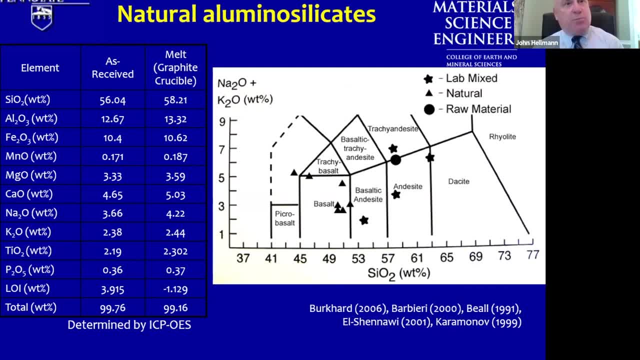 in the roofing product. Therefore these are put back to landfill at very substantial cost, the order of $9 per ton. transportation costs back to landfill. So these materials should be available relatively inexpensively and in massive quantities- millions of tons per year. 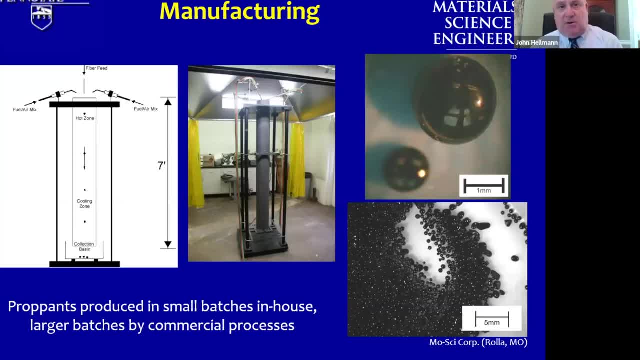 So we procured some of those materials. We transformed them back to the obsidian-like glass that they started as using a flame spheretization approach in the laboratory, resulting in beautiful glass spheres very, very high strength on the order of 600 megapascal. 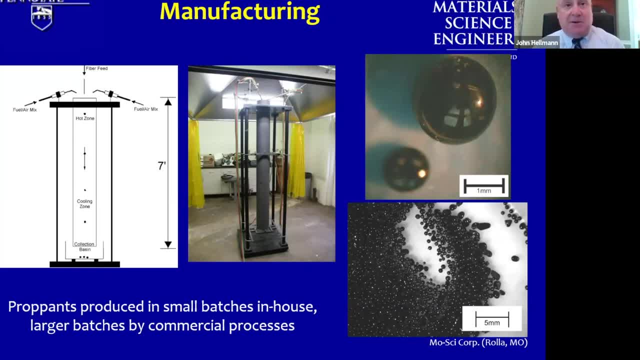 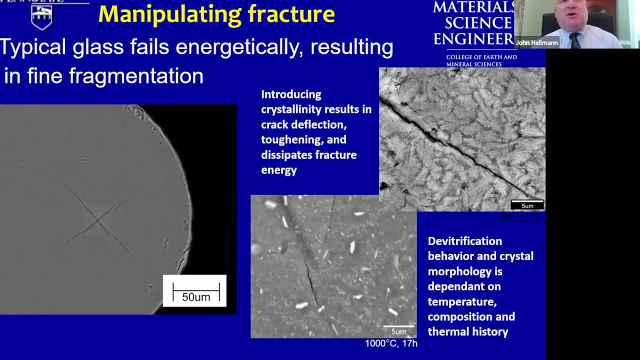 compressive strength, uniformly sized and in massive quantities of three to four teaspoon folds per day. But that was enough to do PhD theses. And what we hypothesized was that if we could take that vitreous material and subsequently de-vitrify it, 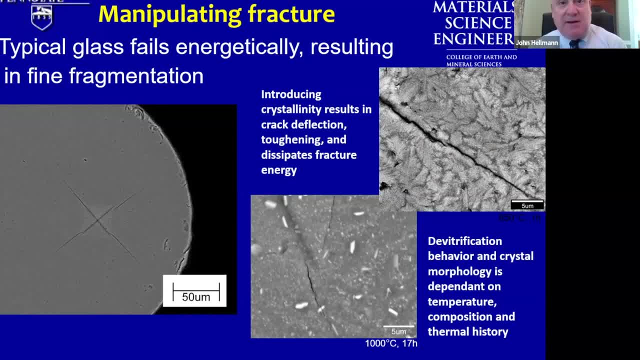 to the crystalline phases that it wishes to be in, that we could alter the fracture mechanisms in such a way to achieve a higher toughness while retaining some strength, and that these beads would fail in that type one failure mode that's desirable for propping. So we did that. We examined, 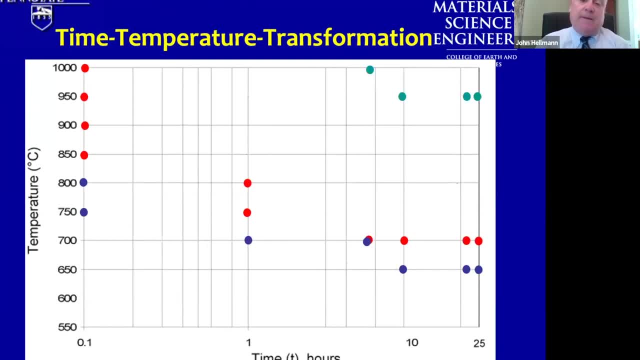 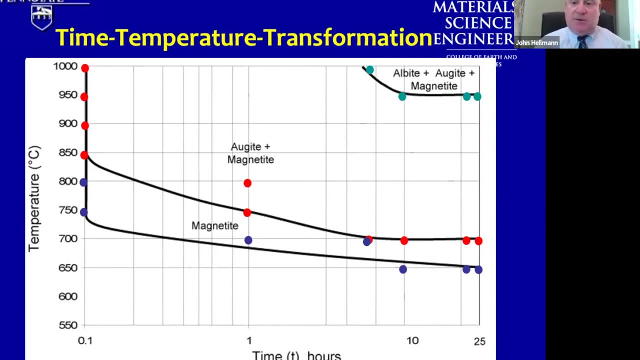 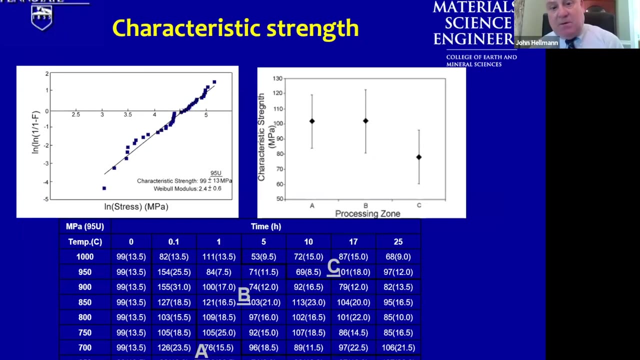 the time-temperature transformation behavior of- in this case, an andesite-based material found out where the different crystalline phase fields were accentuated in time-temperature behavior, manufactured materials in those regions and examined their characteristic strength using the WABL approach I mentioned previously. Characteristic strengths were quite impressive. 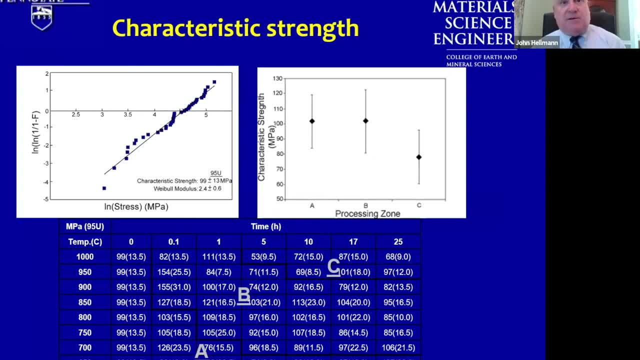 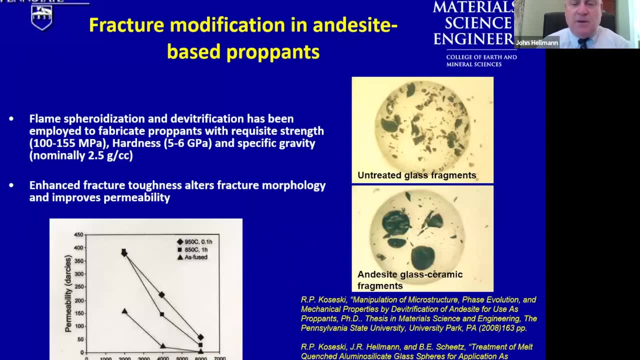 on the order of intermediate strength propants commercially available in the industry- state-of-the-art stuff- and that the material was maximally resilient. So the failure: the fracture was substantially modified after de-vitrification, going from in an untreated glass particle shown in the upper right, fine particulate failure that's. 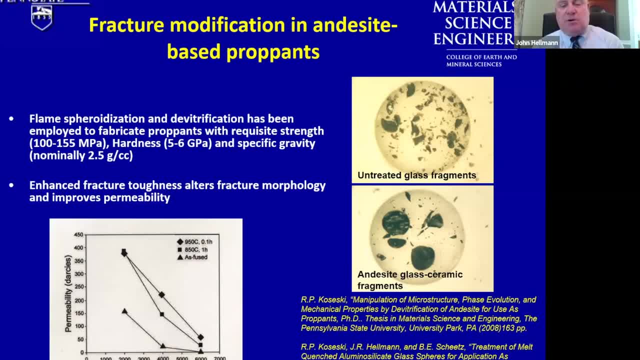 undesirable type 2, to the type one failure: large ceramic particles which still prop. This was then reflected in the enhanced permeability of these materials, which compared very, very well with industrial materials that were still in use, And this was very, very important. And that was the design that we were really focusing on when we were looking at a process that was very, very important to us and the process that we were working on, And that's what we were working on, And that's what we were working on. 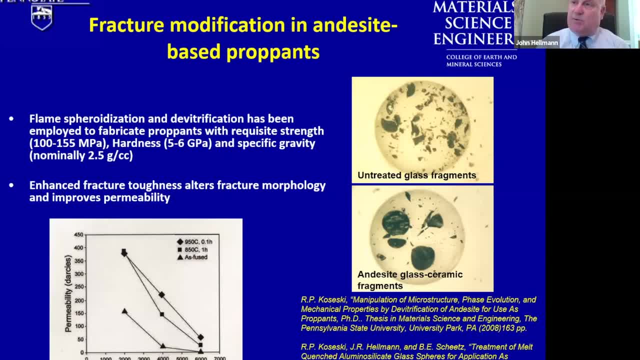 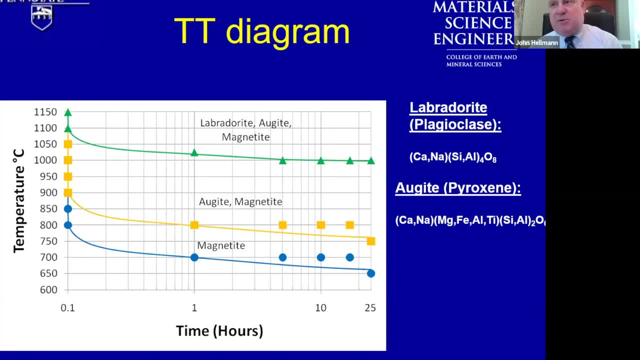 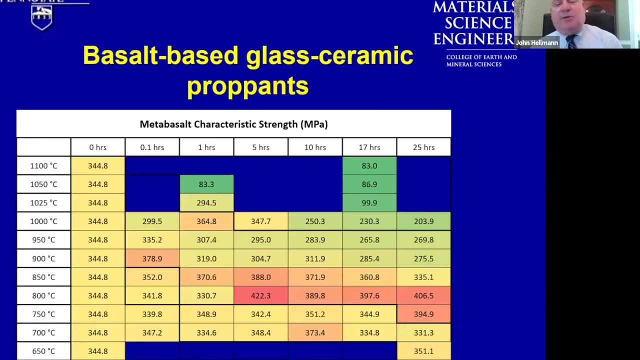 gas industry. We extended this work to metabasalts because that particular mining operation was closer to us and closer to the Utica and the Marcellus shales. We did the same result, or found the same result on time, temperature transformation, And we were able then to map out regions of time. 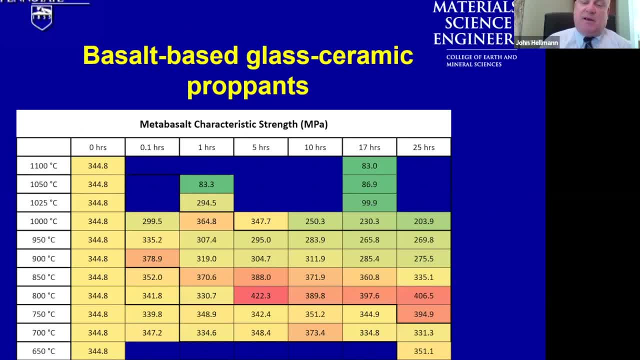 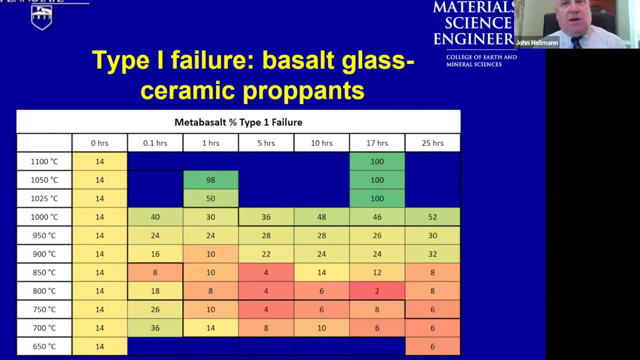 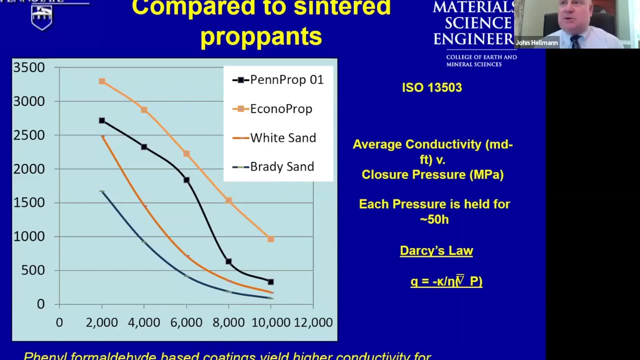 and temperature, which would yield high strength and, at the same time, high type one failure. So we patented this technology and we spun it out for commercialization in a startup company because we felt the material properties would be sufficient for widespread application in the propping industry. We compared these materials using the ISO 13503-2 or API 61. 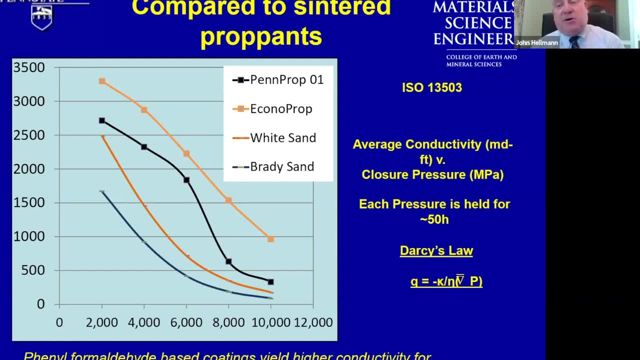 and we found that the material properties were sufficient for widespread application in the. We compared these materials using the ISO 13503-2 or API 61 and we found that the material properties were sufficient for widespread application in the propping industry. We found that these materials 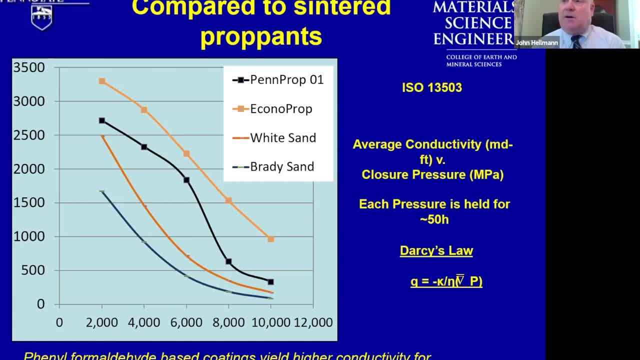 which we are now calling PenProp, which was a trademark name developed by the Nittany Extraction Technology Company, performed very, very admirably well compared to state-of-the-art propens that were readily available at low cost in the industry, and that these materials were performing this way. 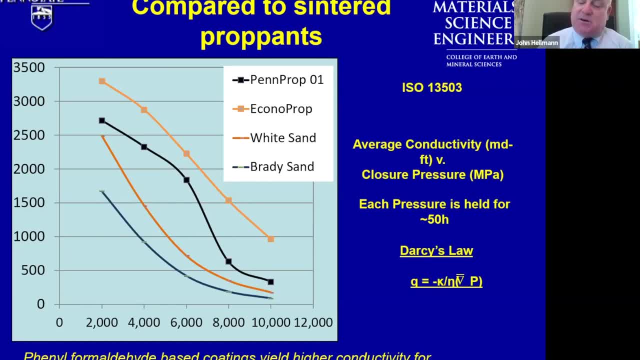 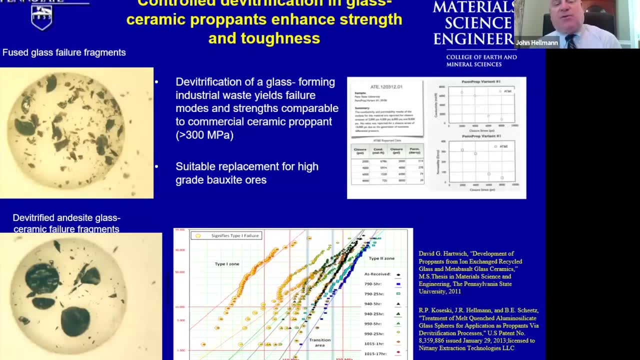 without coatings, The PenProp materials did not perform as well as the Nittany Extraction Technology Company did not perform as well as the Nittany Extraction Technology Company did not need coatings to perform as well as the industrial materials that were available. So this de-vitrification processing allowed us to form a glass ceramic process or glass ceramic. 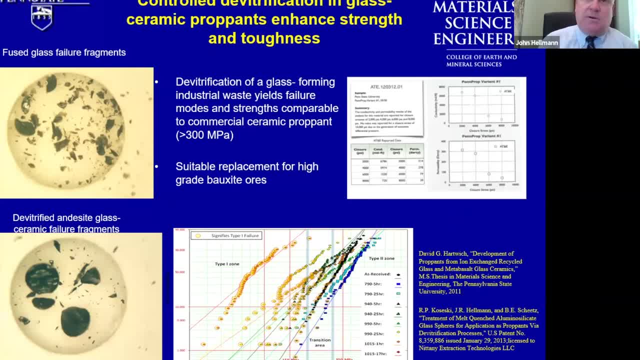 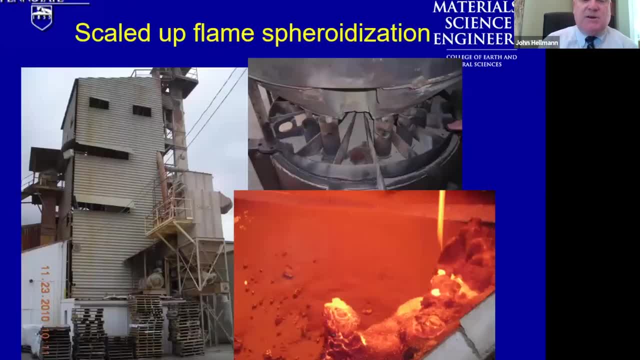 material that failed in type one mode possessed high enough strength and great permeability relative to commercially available materials. So we scaled up to go from the teaspoonfuls per day or week to tonnage quantities per day. So we scaled up to go from the teaspoonfuls per day or week. 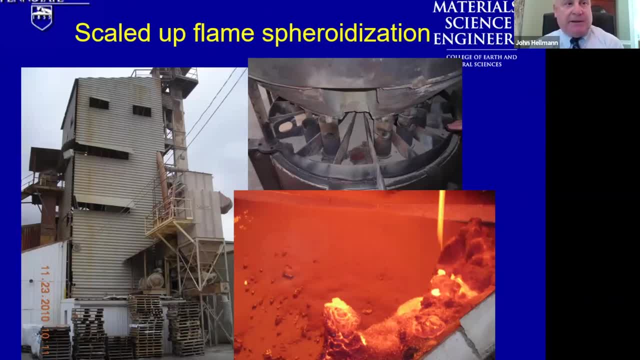 to tonnage quantities per day or week to tonnage quantities per hour. required industrial manufacturing capacity, which we were able to access through a collaboration with A&H Refractories. now Harvest and Walker again. This is a flame spiritization tower that was developed back in the 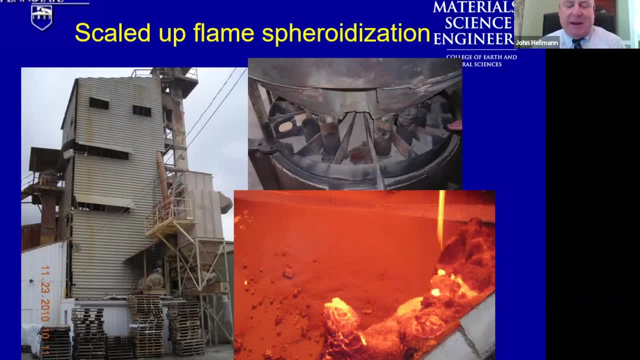 60s by A&H for manufacturing expanded kaolin-based products for insulating refractories manufacturing. Well, we used it to go ahead and do a flame spiritization drop tower approach. much like you would make lead shot for shotguns in which we granulated the metabasalt powders. 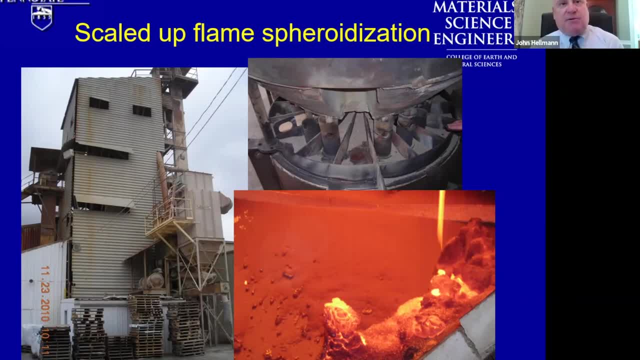 using pan mixing processes to form large granules on the order of a millimeter or so in size and then dropping them through the hopper at the top of the tower. The tower then consisted of 32 radially oriented gas burners- natural gas-fired burners- firing at roughly a million BTU per hour firing rate. 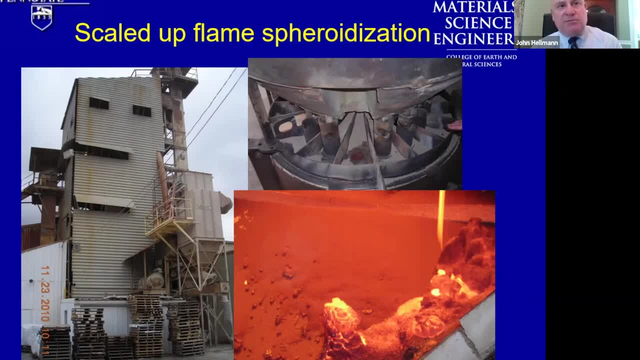 Those particles would melt, fuse, spheridize due to surface tension, solidify on falling down the tower and be collected at the bottom on a vibratory bed and transported out of the furnace in such a way that we could retrieve the materials for care. 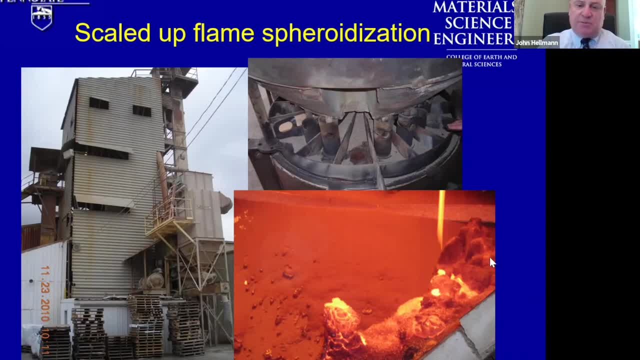 If you look closely at this particular photograph, you'll see lots and lots of vertical striation. That is actually the falling particle rain, the incandescent particles- essentially obsidian-based glass particles- falling at the base of the drop tower. So it was a pretty impressive process and we were able to demonstrate the capability to manufacture tonnage quantities per hour in this fashion. 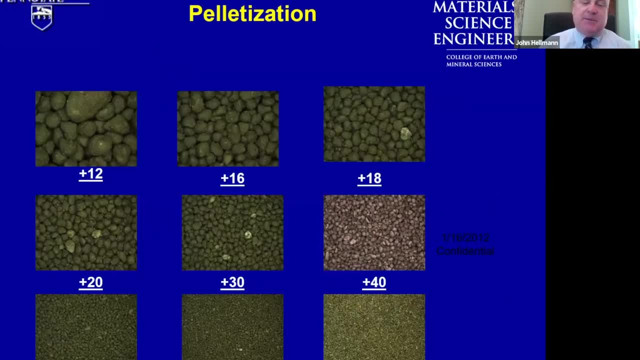 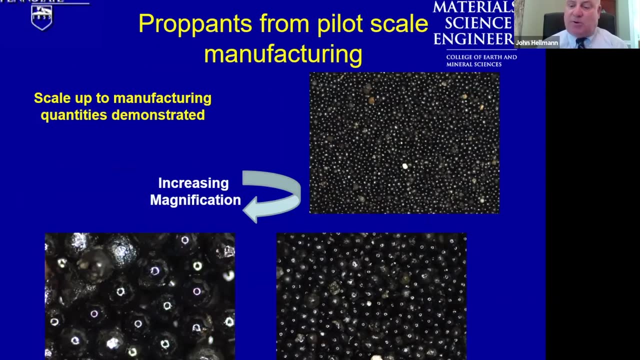 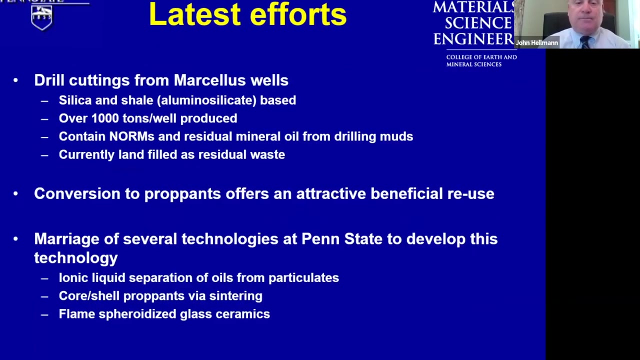 This is a picture of the granules before they were spheridized and after spheridized: Very, very uniform particle size, excellent vitreous particles that subsequently we would heat treat for subsequent testing and use. So our latest efforts have focused on using that technology, on transforming another raw material- drill cuttings- from Marcellus Wells into province. 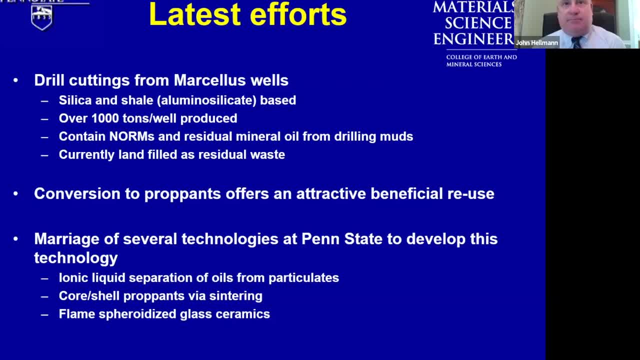 When you drill a well, you basically bore out sandstones and shales from the bore, what becomes the bore, transport them to the surface with your drilling mugs and then dispose of them. These drill cuttings are produced in pretty massive quantities- well over a thousand tons per well. 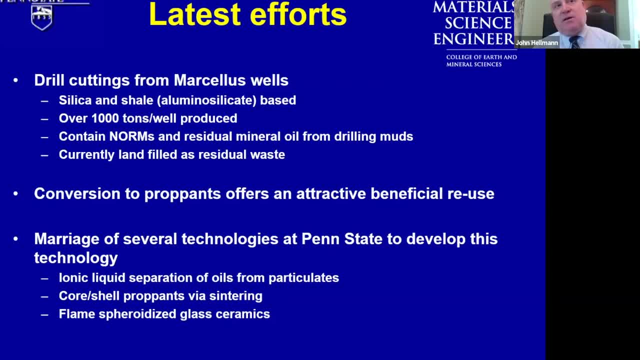 And they contain naturally occurring radioactive fumes. And they contain naturally occurring radioactive fumes. These drill cuttings are experienced physically with materials and residual mineral oils, So when they're transported to the surface they have to be shipped to engineered waste landfills and sequestered as a residual waste. 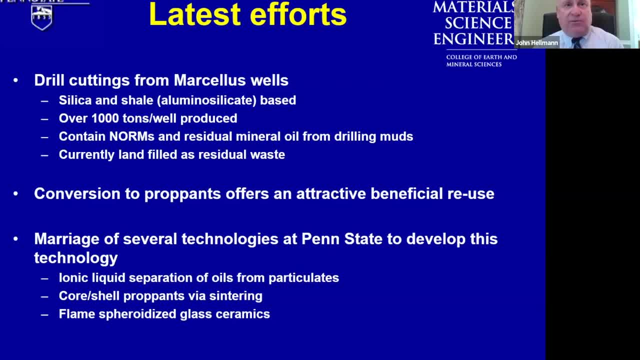 This is a material that costs money to dispose of- on the order of $50 to $80 per ton- and is readily available in areas where you're drilling the wells. This is a material that costs money to dispose of- on the order of $50 to $80 per ton- and is readily available in areas where you're drilling the wells. 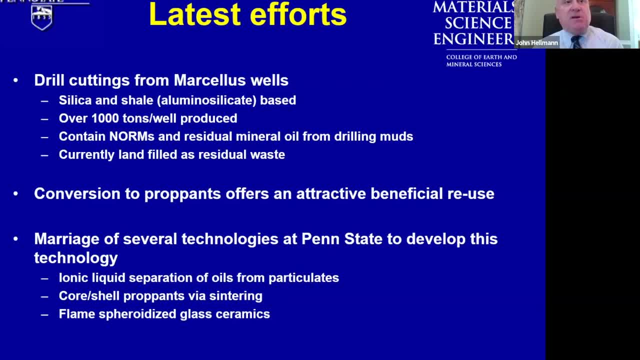 therefore, if we could find a way to convert those materials into you can, And while we're fine, intervene them with the ground, and we- and our research has been successful- drill cuttings into propants and put those propants back into the formations from whence? 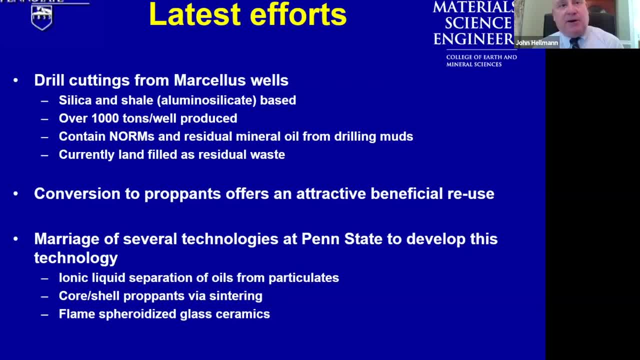 they came, we would experience significant economic and environmental benefits. We felt that we were able to do this by marrying a couple of technologies that were evolving at Penn State at the time, the first being the flame spheretization approach. I've already shown you. 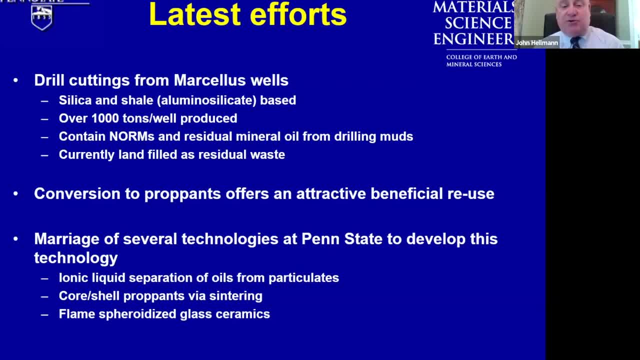 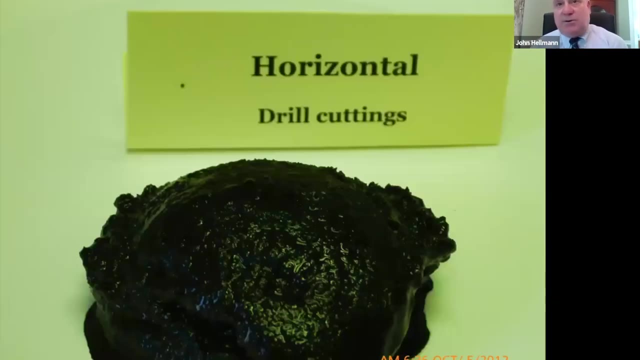 and the second being ionic liquid separation of oils from particulates. This was technology that was being developed to beneficiate tar sands from Canada, to remove the bitumen-based materials from sand and clay particulates that were mined in the tar sand region. The approach that we used was necessary because this is what a drill cutting looks like. 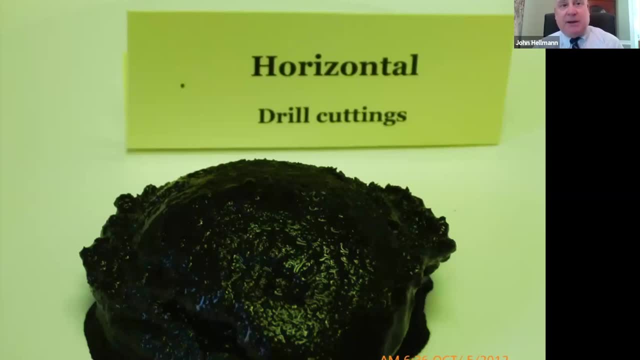 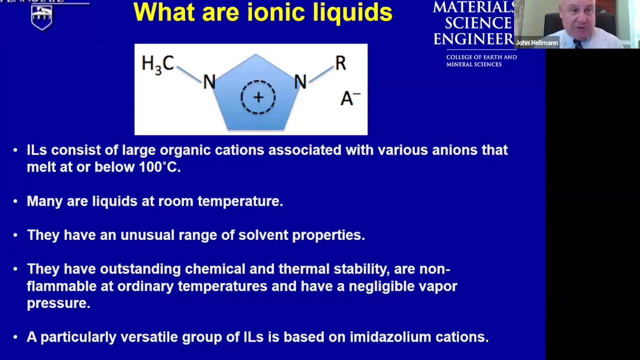 when it comes to the surface, It's a black paste of shale particles suspended in mineral oil and containing other things like sandstone. We need to transform that into a dry powder particle for processing using conventional ceramic processing methodologies. We did it using an ionic liquid separation process that was being 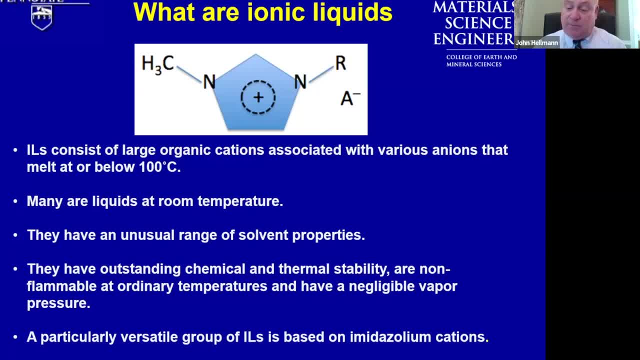 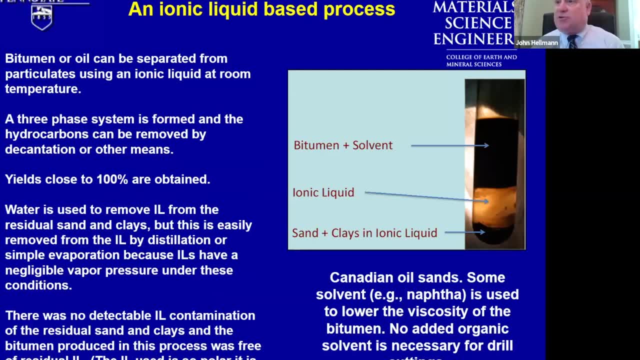 developed at Penn State for the tar sands. This test tube on the right shows the result that you get when you use ionic liquid: separation of bitumens from ceramic particulates like clay and sand. The bitumen and some solvents are shown in the upper layer, the ionic liquids are in the middle and then the sediment at the bottom. 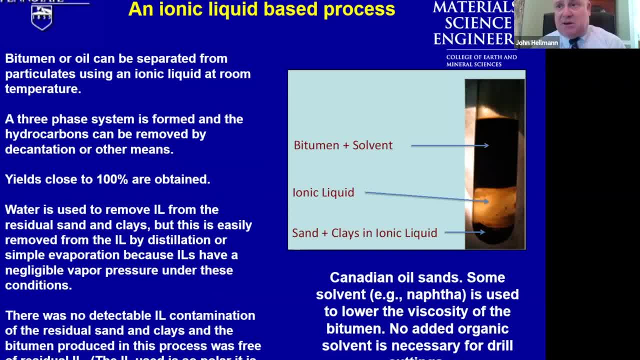 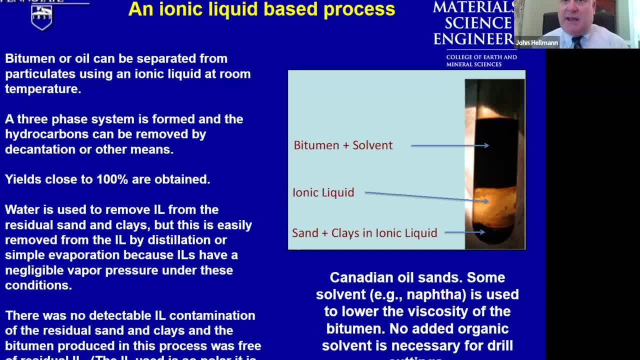 we can extract its surface. It's also desirable, but we would be extracting the sand and clay and using that. Fortunately, the ionic liquid separation process works well on drill cuttings. Ionic liquids can be separated from the powder particles by a water wash, which is great. 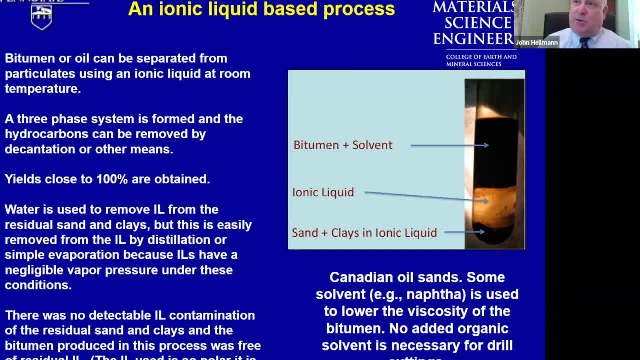 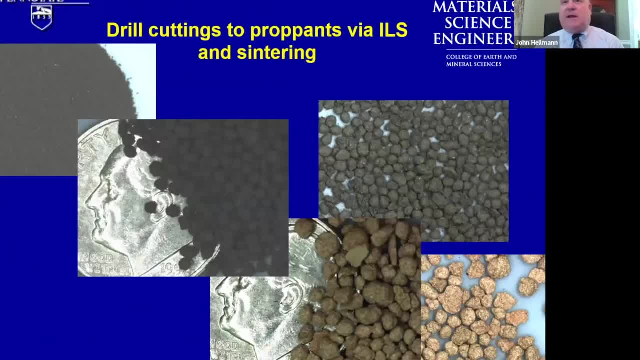 environmentally sensitive. The ionic liquids are recyclable and containable, also environmentally desirable, and so we were able to manufacture aggregates from the drill cuttings that were produced from the ionic liquid separation process. These are showing some of the aggregates before and after centering. This is preliminary work demonstrated that we're able to make aggregates. 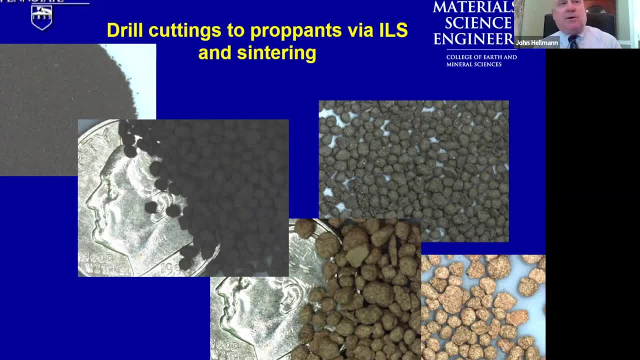 that are moderately high strength should be useful for aggregates for construction as well as for propping gas wells with more development. More development means that we need to enhance the centering kinetics. so back to our doped centering studies from earlier in this presentation. 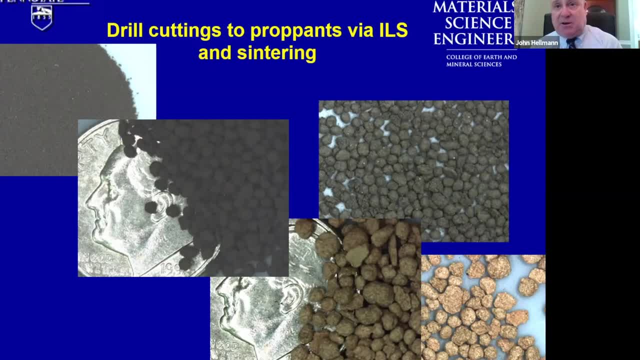 and that's where the approach is. Because these are such high silica content compositions, we need to flux that silica to promote liquid phase centering. but we can also flame spheridize these materials as shown here. These are proppants made. 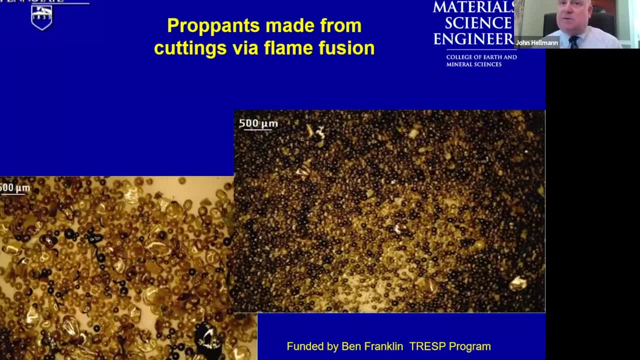 for the production of aggregates, and so we're able to make aggregates that are moderately from drill cuttings after ionic liquid separation, aggregation and passing through our flame tower, We're able to make quite uniform, highly vitreous beads which subsequently, once 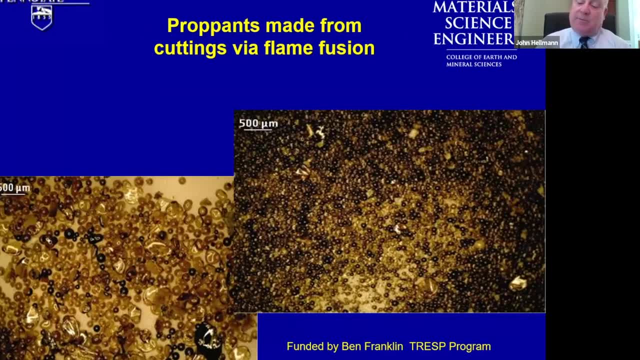 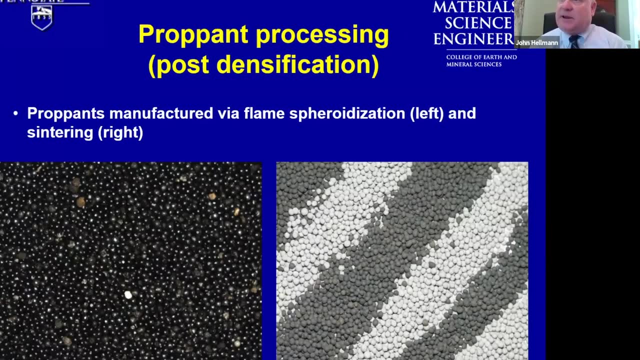 de-vitrified will perform like we demonstrated with the metabasalts and andesites. So the proppant processing technologies that we developed work with drill cuttings. On the left, you see vitreous beads. On the right, you see de-vitrified beads On the left, you see. 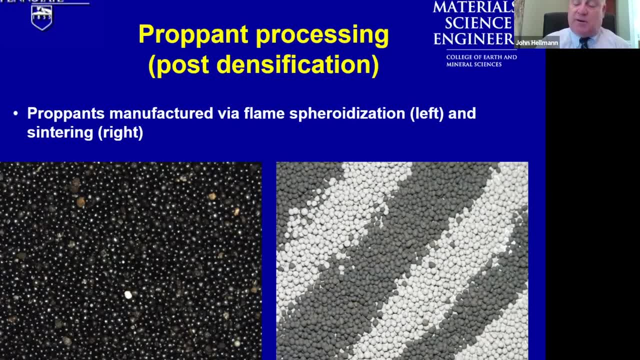 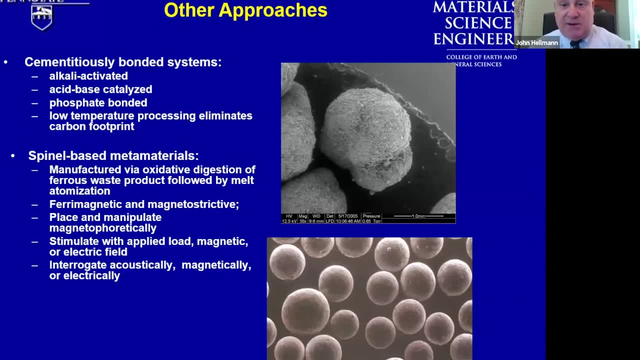 de-vitrified beads made by flame spheridization. On the right you see commercial proppants manufactured via centering. There are other approaches to densifying these materials: Cold centering and cementitiously bonded systems. both work. We've demonstrated that in other work. 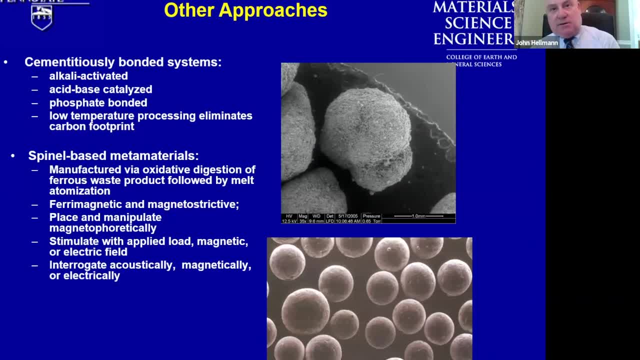 that we can achieve moderate strength particles from some of these raw materials without requiring centering cycles. Hence we're able to make these materials. No use of hydrocarbons, no production of CO2.. Similarly, we're looking at other byproducts of industrial processes for proppant applications. 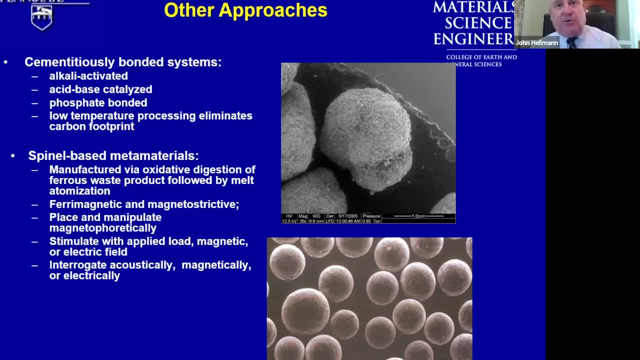 One is the swarf that's left over from the manufacturing of ferrous-based ball bearings. All right, the swarf, or grinding powders if you will, can be transformed back to ceramic using a flame atomization process. This can be done by using a flame atomization process. 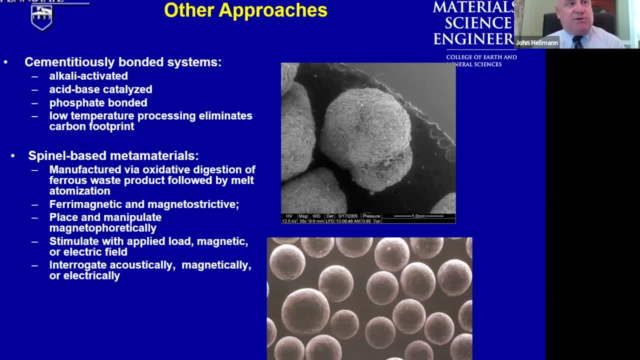 This can be done by using a flame atomization approach which forms first wustite, which is highly fluid and spheridizes in the flame due to surface tension and then later in the flame plume. by adjusting oxygen, partial pressure can be converted to magnetite. Magnetite is desirable. because it's magnetostrictive, which means that in the presence of a magnetic field it changes shape. And if you put that material in an alternating magnetic field, it'll change shape in an alternating fashion, hence vibrate If it vibrates. 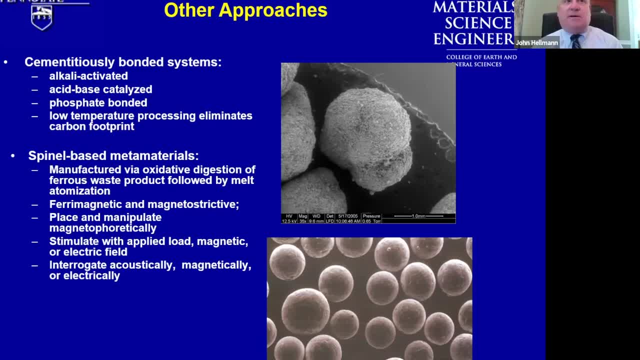 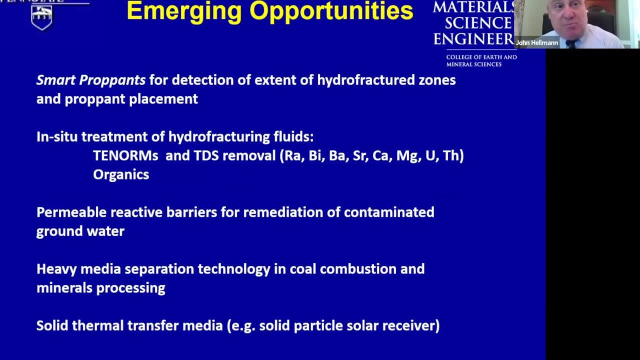 you can detect the material acoustically. You can also emplace the material magnetopheretically and you can stimulate it using magnetic and or electric field. So this brings us into the world of a whole new proppant application that we term smart proppants. 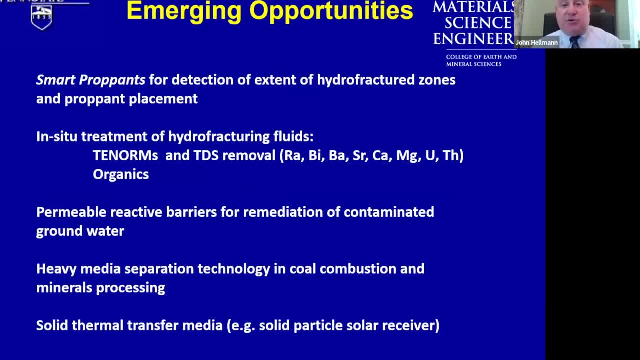 and we're replying a fair amount of our attention right now. Smart proppants would allow us to not only place the materials using magnetopheretic stimulation, but also detect them later on, once they're in place, to understand the magnitude or the size of a propped hydraulically fractured 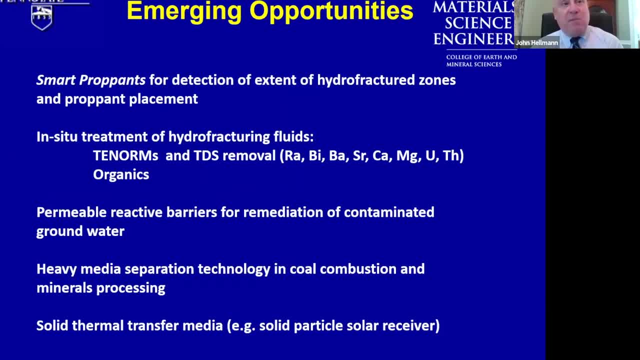 shale deposit. That's important for many, many reasons, ranging from understanding how the production of the well will change over time, to also understanding how the production of the well will change over time, to also understanding just exactly where is your well with regard to. 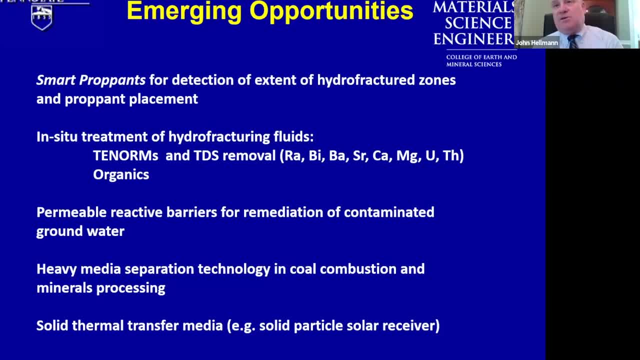 private property, boundaries and the like. These materials may also have an application for in-situ treatment of hydrotracturing fluids By substitution of other transition metal ions instead of iron. we believe that we can make these things moderately catalytic for removal of total dissolved solids, as well as potentially T-norms, and possibly also perform well as permeability. So this is a very good example of how we can make these things moderately catalytic for removal of total dissolved solids as well as potentially T-norms, and possibly also perform well as permeability. So this is a very good example of how we can make these things moderately catalytic. 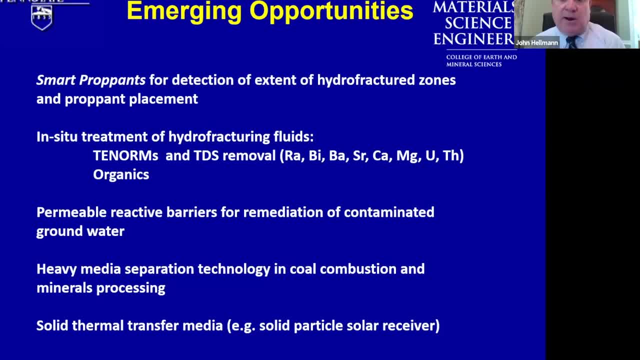 for removal of total dissolved solids as well as potentially T-norms, and possibly also perform well reactive barriers for remediation of contaminated groundwater. They're also useful as heavy media for heavy media separation in coal grinding and minerals processing. Those are desirable characteristics that we could develop further. and what goes? 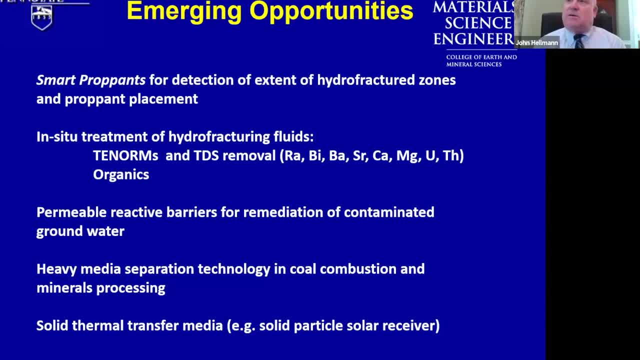 around comes around. These materials now are inexpensive, spherical refractory colored. We can color them, We can make them anything you want. pretty much We can make them highly absorptive in the solar spectrum. So here we are, back to solid thermal transfer media. So to summarize, it's been an 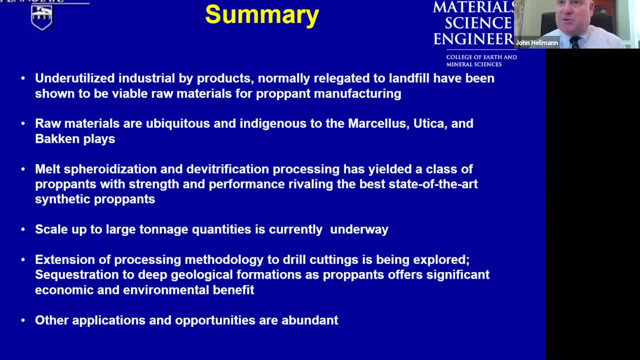 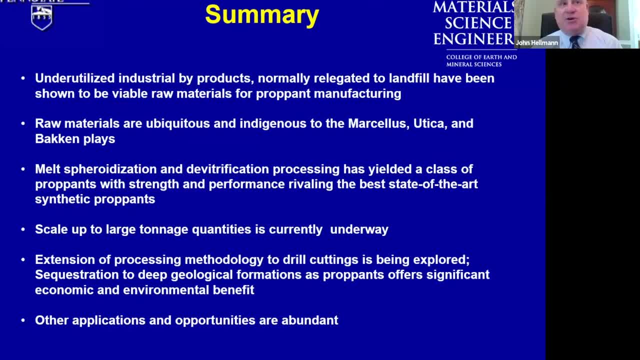 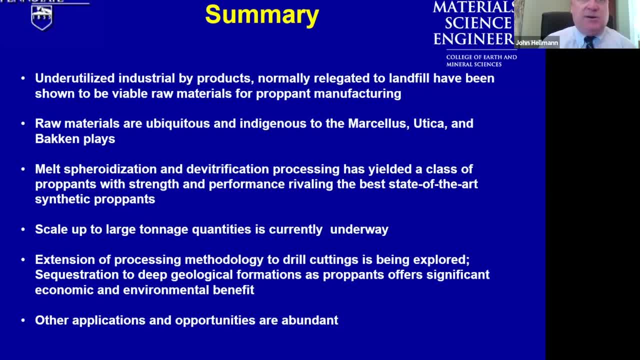 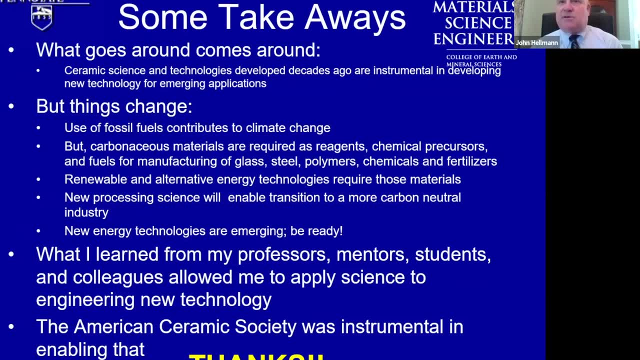 Other applications and opportunities are abundant. It's only a measure of how creative do you wish to be. So some takeaways Again. what goes around comes around. The ceramic science and the technologies that were developed decades ago were employed in these studies. here to 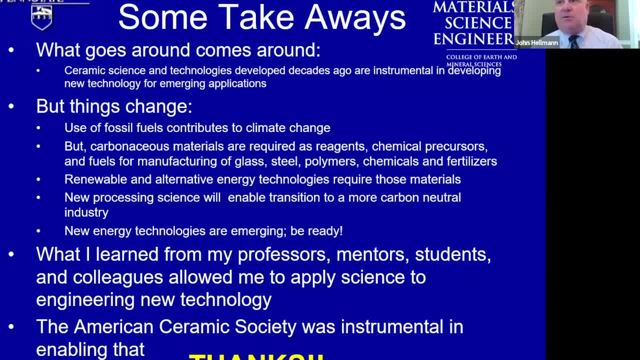 how to manipulate the properties of a material. by manipulating the processing characteristics, We developed a suite of profit materials that are instrumental in enhancing the ability to retrieve gas and oil from unconventional deposits- the natural gas shale boom, if you will, which created energy independence. 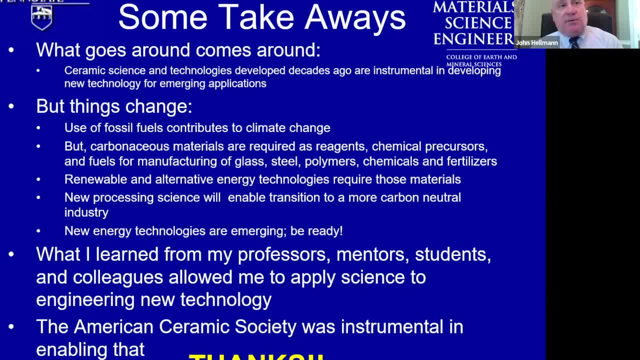 for the United States 15 years ago. However, things change. The use of fossil fuels like natural gas contributes to climate change. Lots and lots of evidence that burning fossil fuels- creating CO2, changes the temperature of the earth in a localized sort of way, affecting climate change. 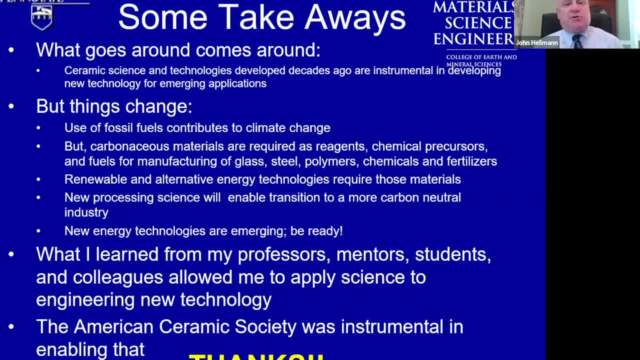 and that this is an issue that is going to be pushing us towards becoming a society with a better, lesser carbon footprint. But carbonaceous materials derived from hydrocarbons are still going to be required in our society, and that's because they're reagents. 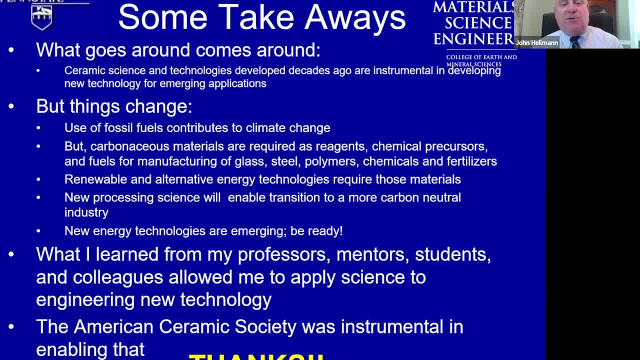 they're chemical precursors and they're fuels for the manufacturing of glass, of steel, of polymers, of chemicals, pharmaceuticals, fertilizers, food. All of these things sustain our life And that the renewable and alternative energy technologies that are evolving, which will supplant some of the hydrocarbon usage in the future, are going to require the use of hydrocarbons to enable them. 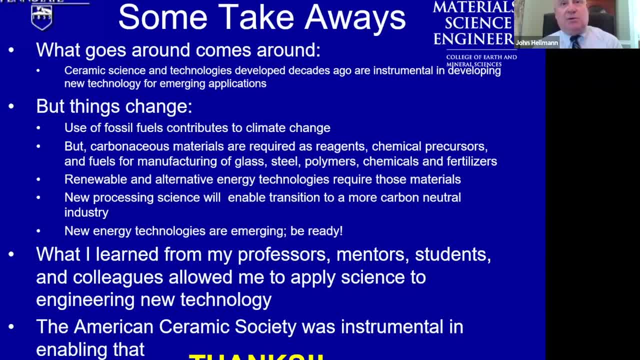 We have to manufacture these materials to build the solar turbines, the hydro turbines, the solar cells and so on. So we need to develop new processing science, New processing science which will enable us to do things like center at lower temperatures and not need fuels, not need to burn fuels for process heat and so on, in order to manufacture ceramic and other materials of sufficient quality to enable continuation of our current lifestyle and advances in the future. 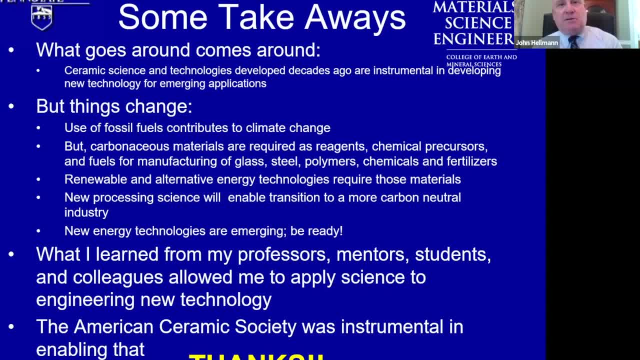 This is a whole area that probably is right now under exploitation. Green manufacturing on steroids. And beware, there are new energy technologies on the way. It's going to change the landscape. You can't pick up a newspaper and not see an article on the current fusion. ears, the people who are working on fusion. 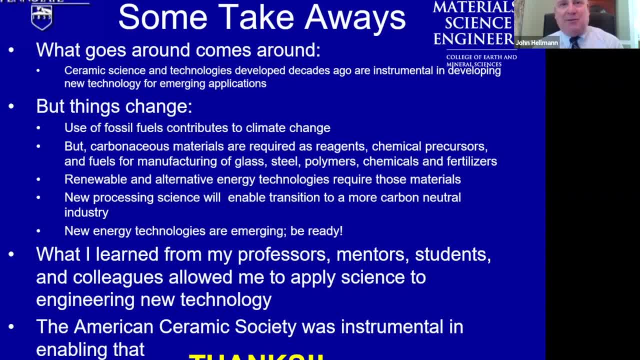 And it's a broad brush of society, quite frankly. And fusion is on our near horizon. Fusion will enable us to generate electricity with a very, very small environmental impact, if any. The issue is it's going to require advanced materials.